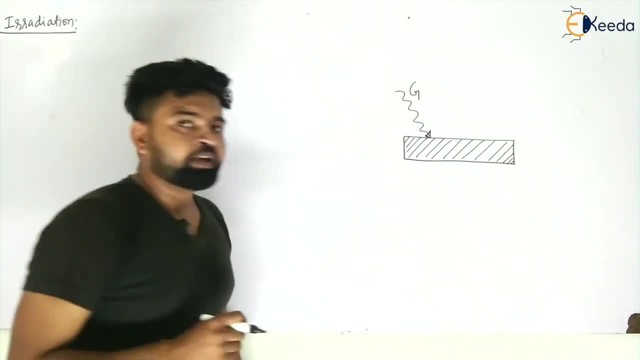 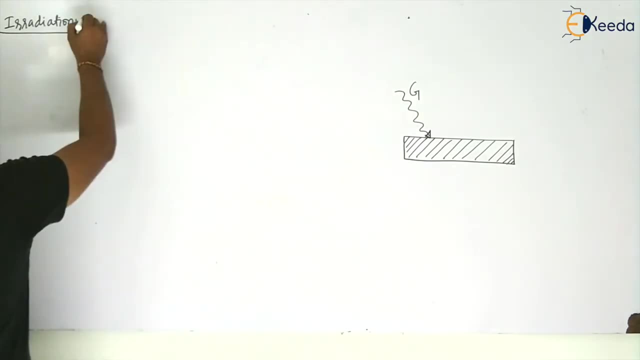 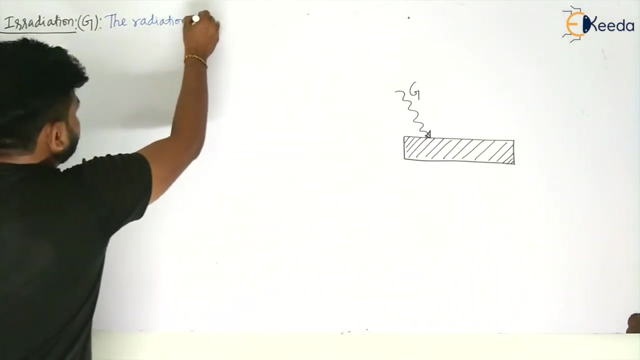 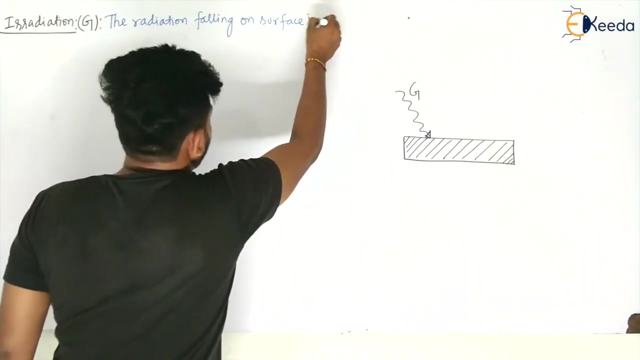 Let us say this is represented by G. So the radiation which is falling on the body is called as your irradiation, and that is defined by G. my dear students, G, The radiation, the radiation which is irradiation falling on, falling on surface, on surface, is called irradiation. 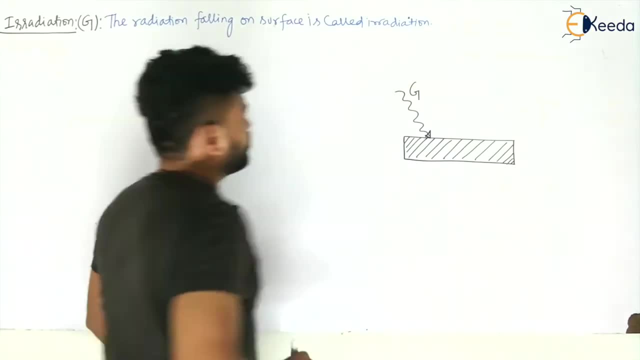 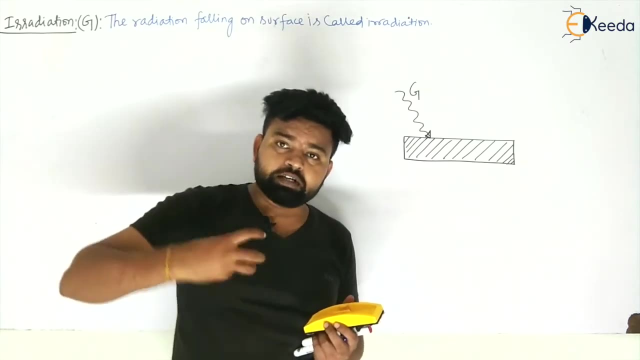 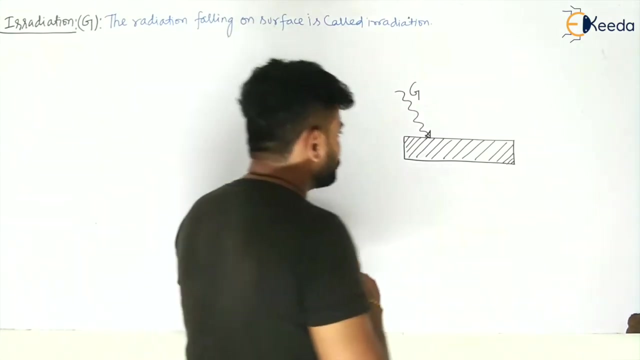 Irradiation, my dear students. Okay, Now, maybe some radiation is emitted. Some radiation is emitted like some is falling on the body and some is like emitted by the body. Okay, Or emitted or reflected by the body. So the radiation leaving the surface. 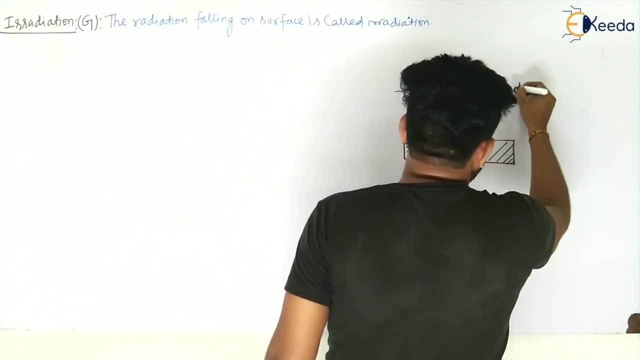 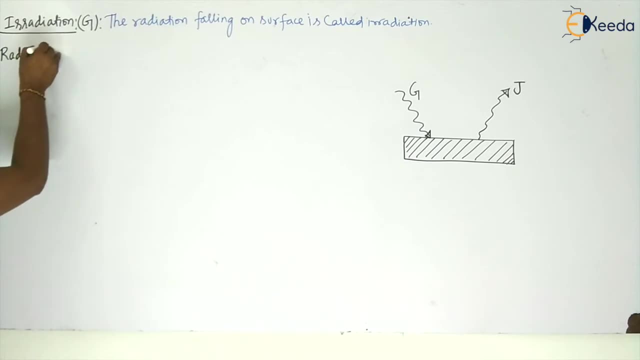 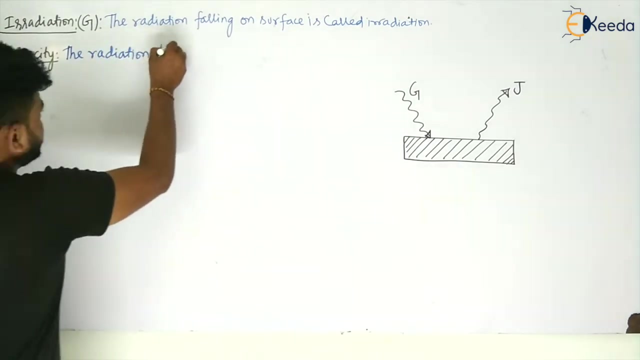 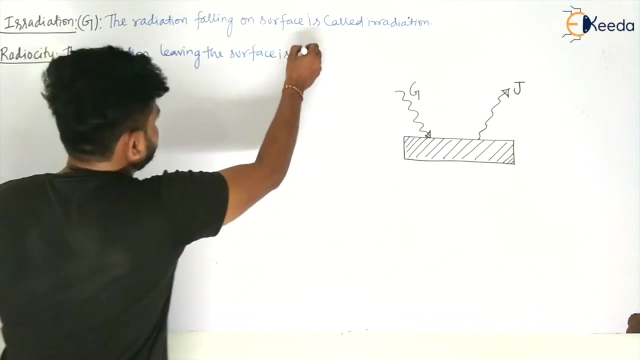 So the radiation leaving the surface is represented by G and that is called your radio city, my dear students, Radio city. So what is radio city? The radiation leaving the surface, Leaving the surface, is called the radiation Leaving the surface, Surface is called radio city, my dear students. 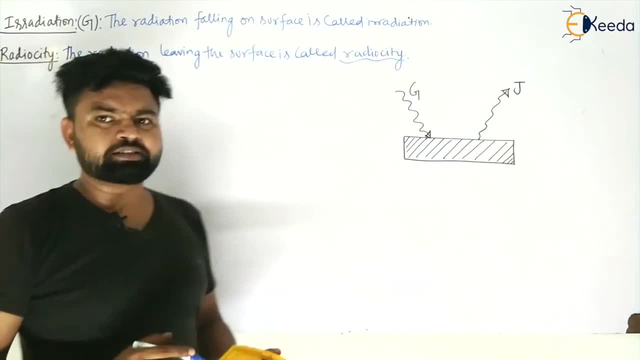 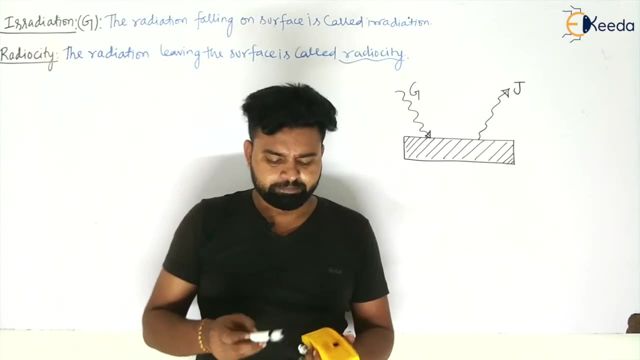 Radio city, So how we can see the radiation which is leaving the surface. So let us understand this concept carefully. Let us say: I have a surface, I have a surface. Let us take, I am taking this surface. Okay, 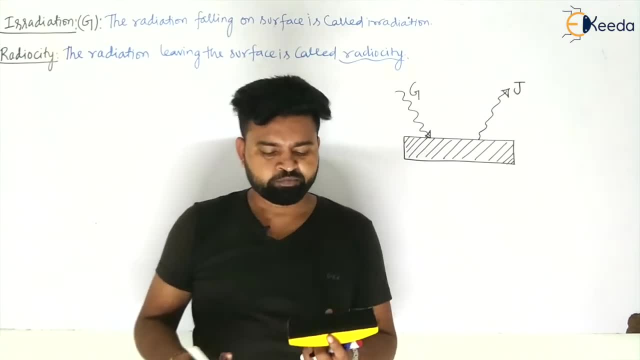 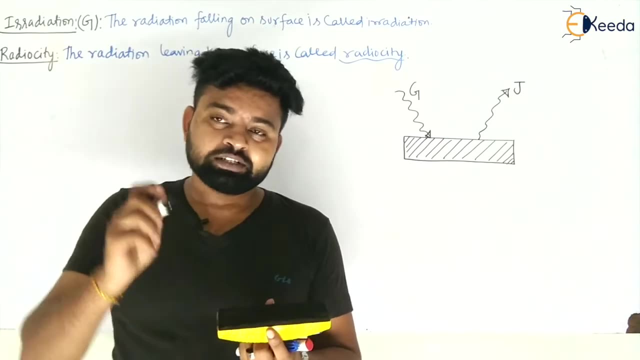 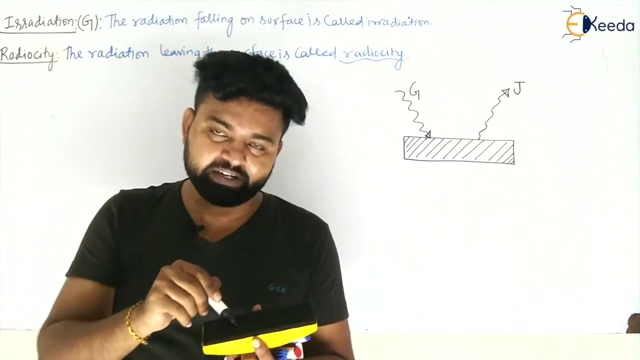 That is my favorite, Okay, I am taking this to be like my surface. So some radiation is emitted by this surface, Okay, And also some radiation which is coming out from the body may be reflected from this body, or coming from outward may be reflected by this surface. my dear students, 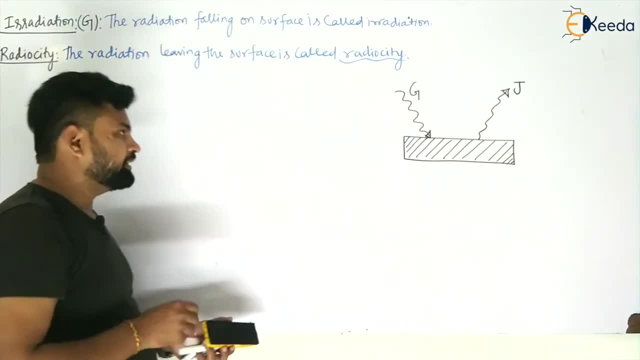 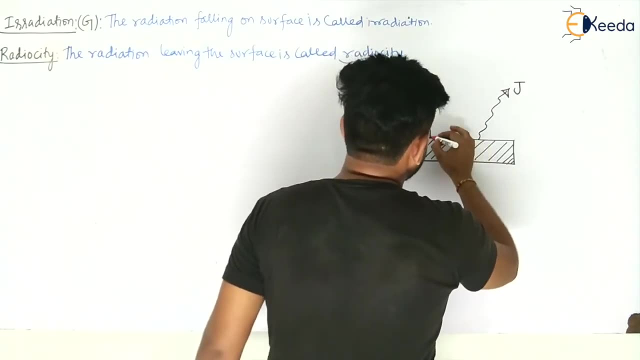 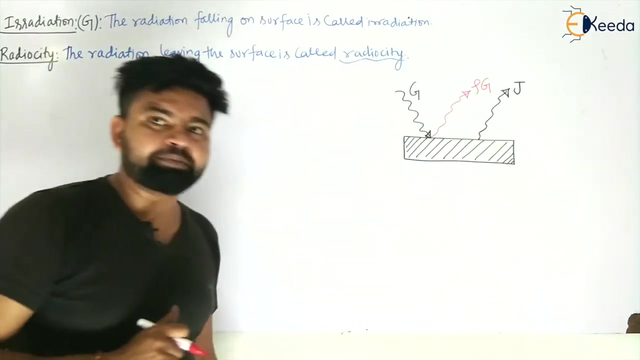 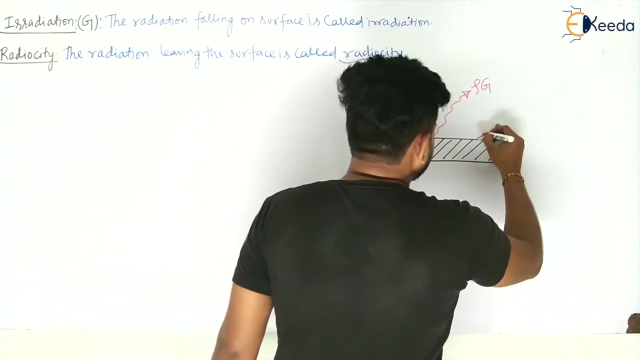 So this can happen, Then the radiation which is coming to the body can be reflected back, Can be reflected back. That will be your rho G. And also, there can be possibility that some radiation may be emitted by the surface. And what will be this radiation, my dear students? 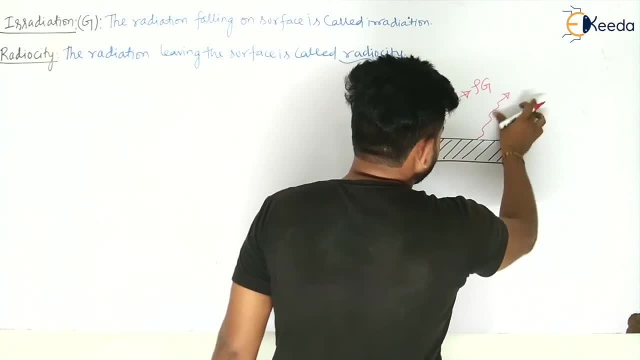 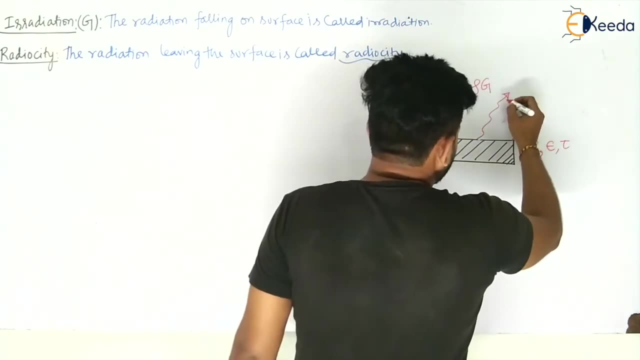 This will be E into, That is emissivity of that surface, If it is having some reflectivity, Some emissivity, Some transmitting, my dear students, So what will happen If this is having some emissivity? So this will. 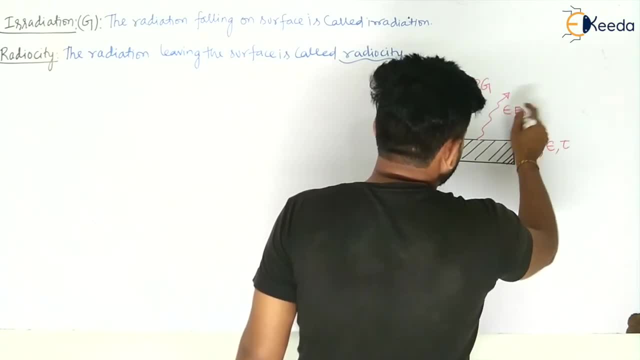 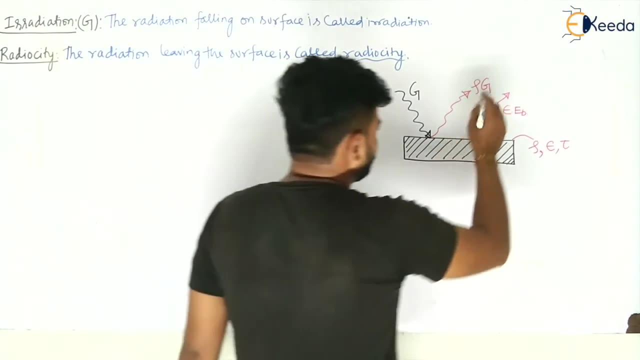 It will also emit some radiation that will be equal to E into E B. my dear students, Just a note. So what will be the total radiation which is leaving the surface? So the total radiation which is- I am calling that radio city. 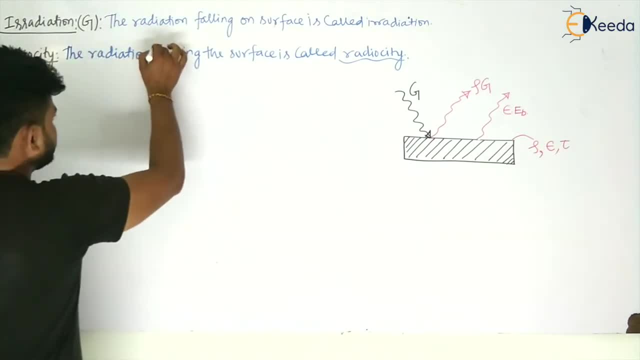 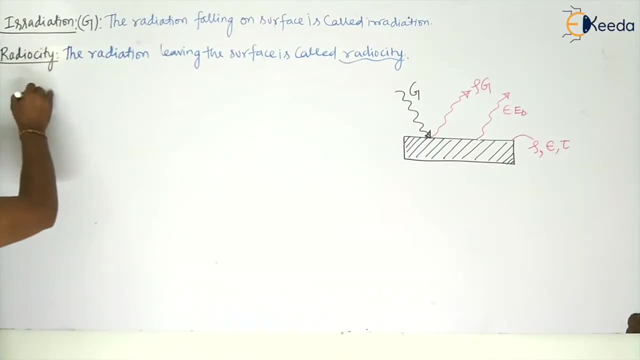 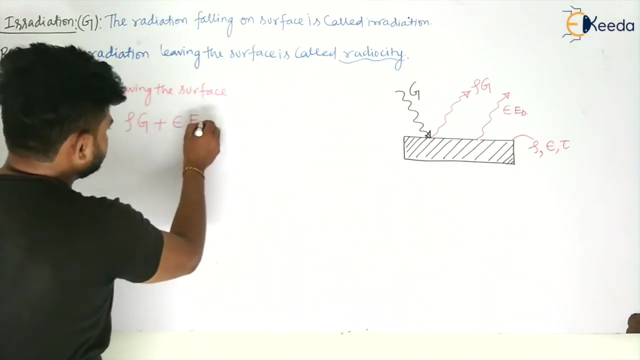 So the total radiation leaving the surface, Total or we can say the radiation leaving the surface. So now, total radiation leaving the surface is equal to how much? So this is defined by J and this will be equal to nothing but rho into G, plus epsilon E into E B. my dear students, 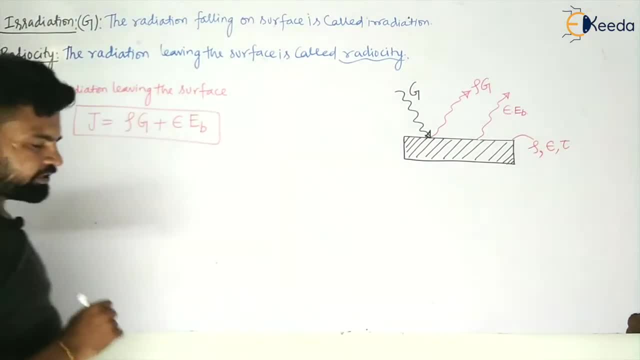 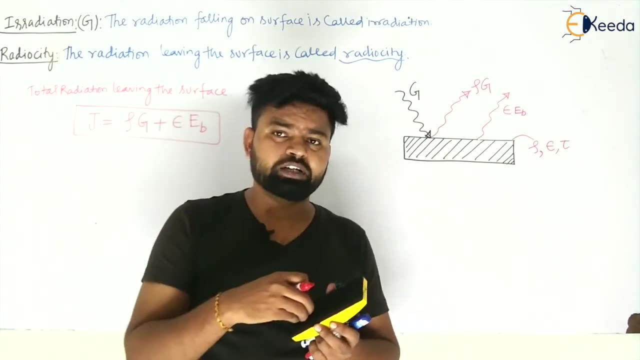 So this will be a total radio city for the body, For the surface. This will be for the like for the. this surface, This is some reflecting and this is also emitting some, So the total radiation which is coming out from this surface will be what 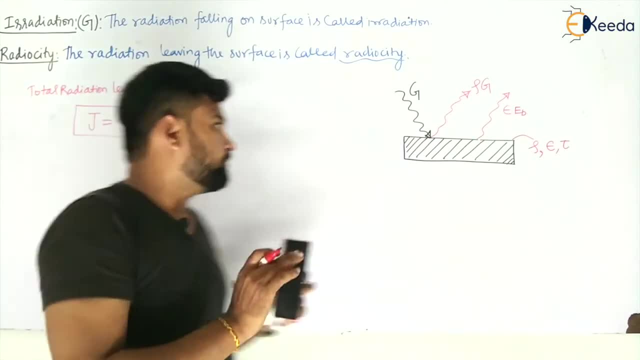 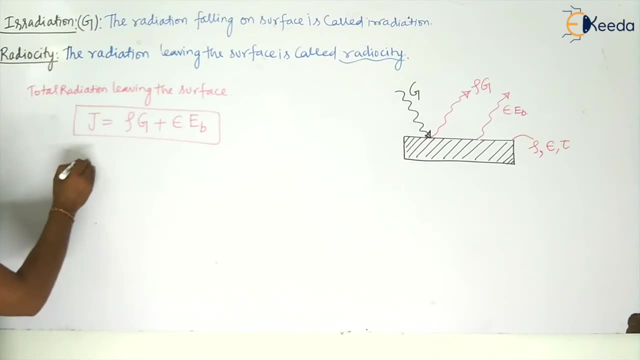 Rho, G plus E into E B. Why? Because that is also emitting and reflecting. Okay, So now can I calculate the value of G from here? Yes, What will be G? So G I can calculate. This will be J minus E of E B. 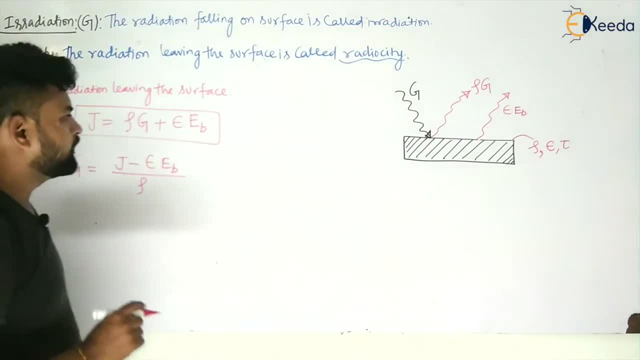 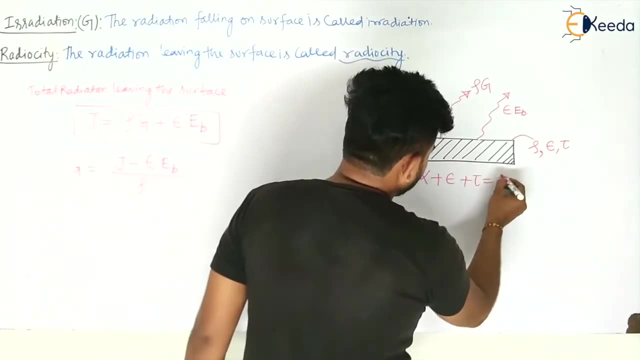 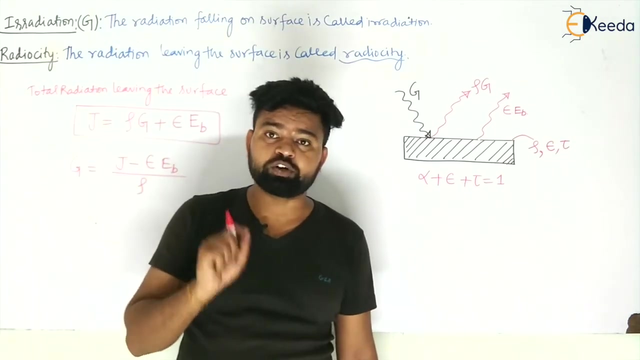 Divided by rho. Divided by rho, my dear students. So I know that alpha plus E plus tau is equal to 1, my dear students, And most of the times we will be dealing about the opaque surfaces, that is, solids and liquids. 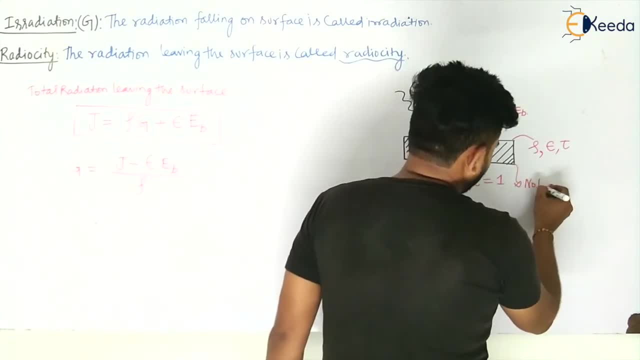 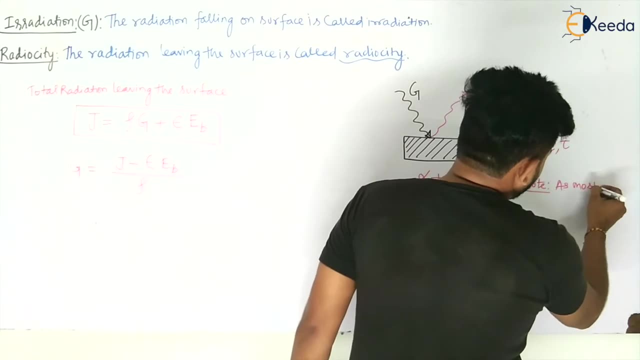 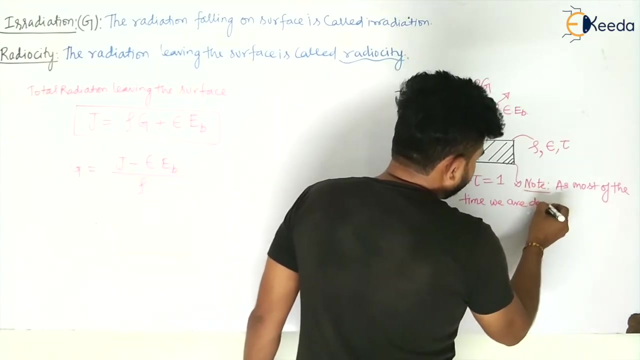 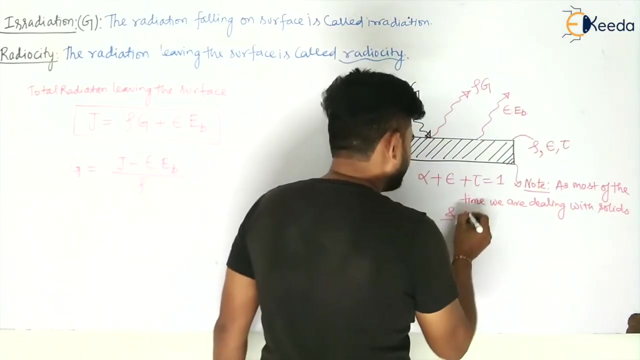 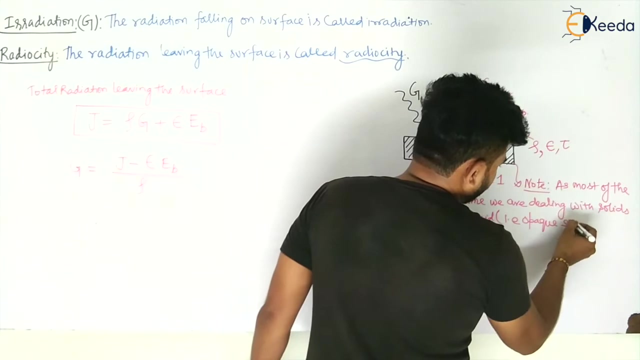 So as- let us take it not as we are most of the time, As most of the time, Most of the time, we are dealing with solids and liquids. Solids and liquids, that is, that is, opaque surfaces. Opaque surfaces, that implies tau will be equal to 0, my dear students. 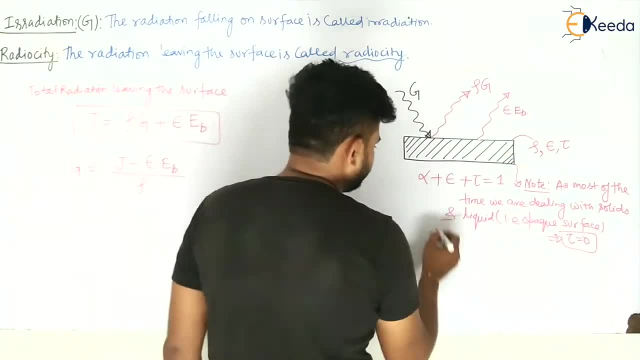 That is transmitting will be equal to 0, my dear students. Okay, So this is rho for this case. So what we will be left with, We will be left with That is not alpha. That is here, your rho, my dear students. 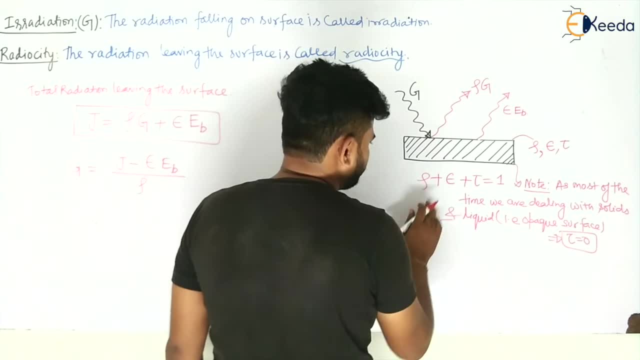 So we will be left with what: Rho plus alpha plus tau is equal to 1.. So that is equal to 0. But in our case, so we will be left with, rho plus alpha is equal to 1, my dear students. 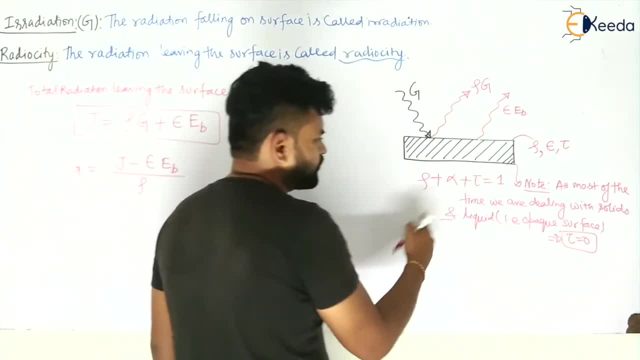 So from Christoph's Law, can I put that alpha is equal to E? from Christoph's Law, all the times I used this step from 1 to E. This one will be V. This one will be X If the equation is I plus O of P. 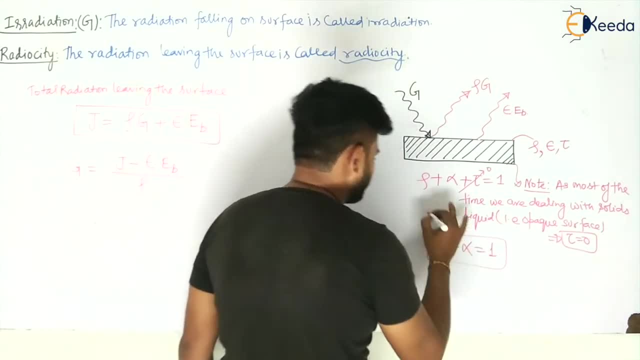 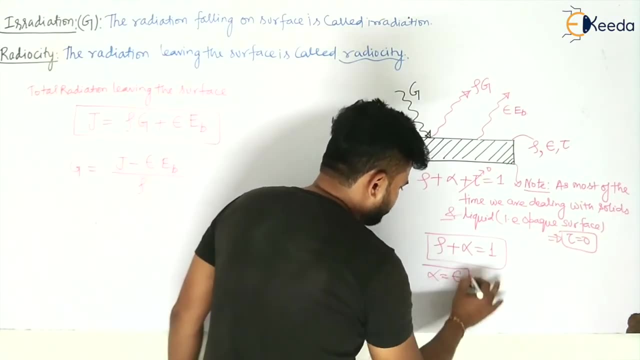 This is I minus A. This is an operator. We will create The operation. if I am not abut Here, I will be. remove all this. That is one of the variables. can I calculate, can I put that alpha is equal to E from Christoph's law, from Christoph's? 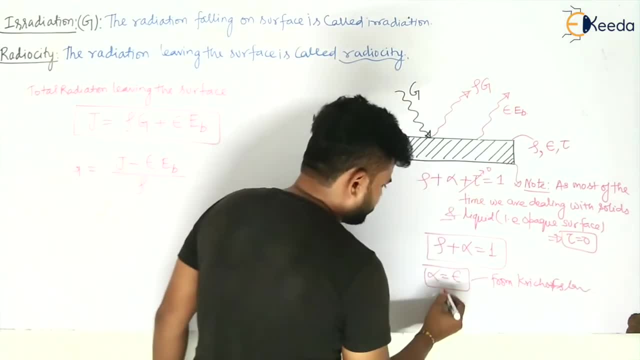 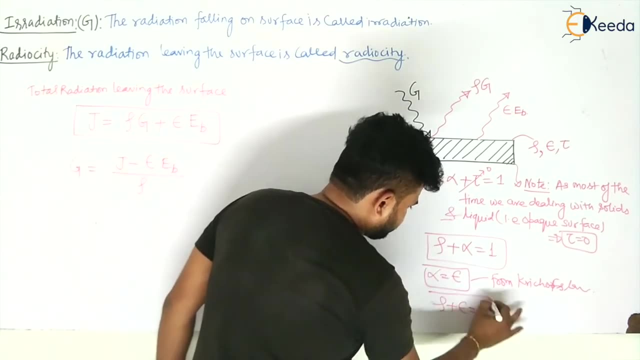 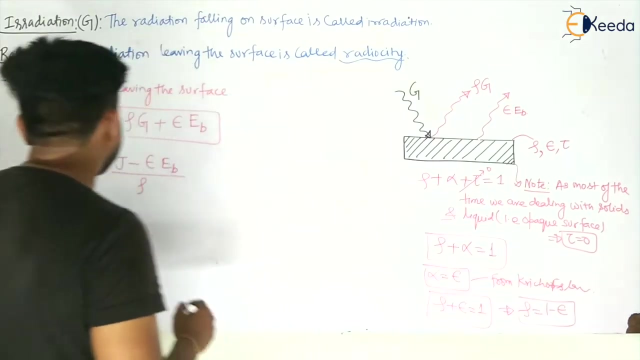 law, Christoph's law, my dear students. so alpha will become equal to E, so this term will become alpha. rho, that is rho plus E, is equal to 1, so can I have the value of rho? so this will become 1 minus E. my dear students, that is epsilon, so this will become. 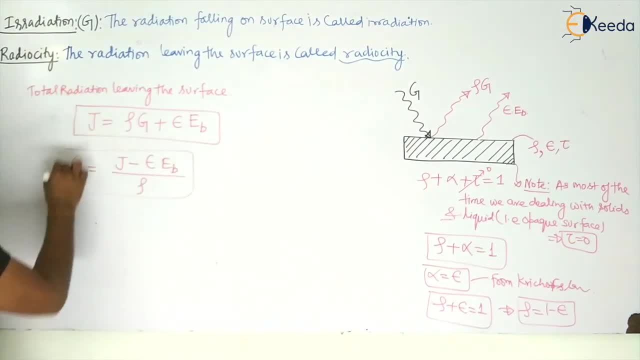 so I will put the value here in this equation, what I will have. let us see. so G will become equal to J minus E of E, p divided by 1 minus E, 1 minus E. so now I have the total radiation. 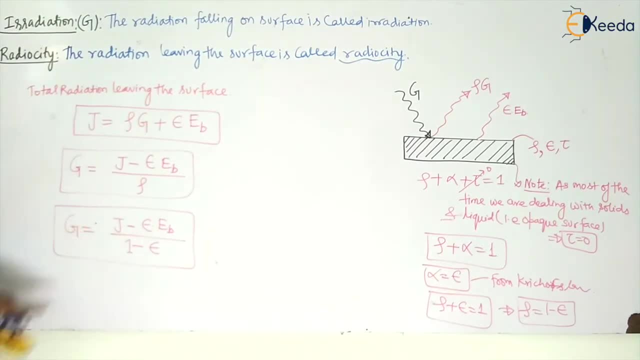 which is falling on the surface. now I have the total radiation which is falling on the surface, my dear students. so let us take this equation, so let us calculate the net radiation here. Let us take the heat exchange between the two surfaces, between this surface, my dear, 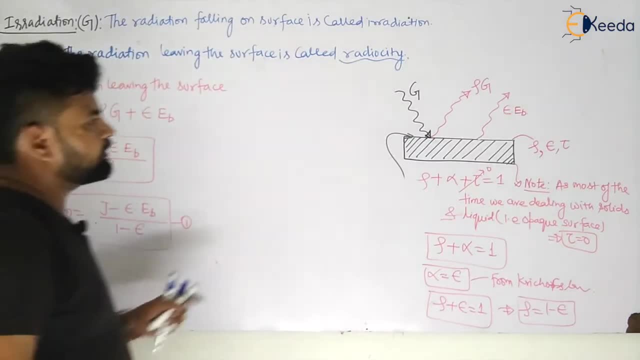 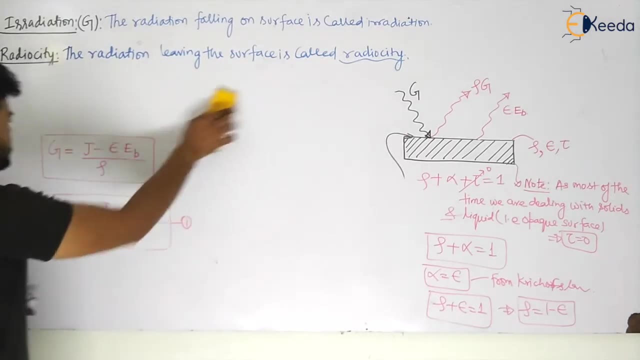 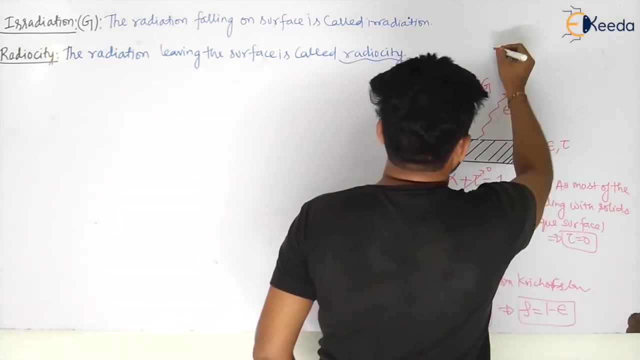 students, what will be this? let us see. so the net radiation with particular surface will be given by what? let us see, so let us calculate the net radiation, my dear students. so let us put this equation there, so that you will remember. so this will be G or J. 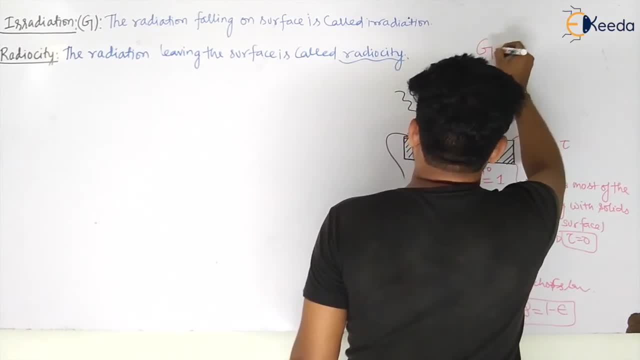 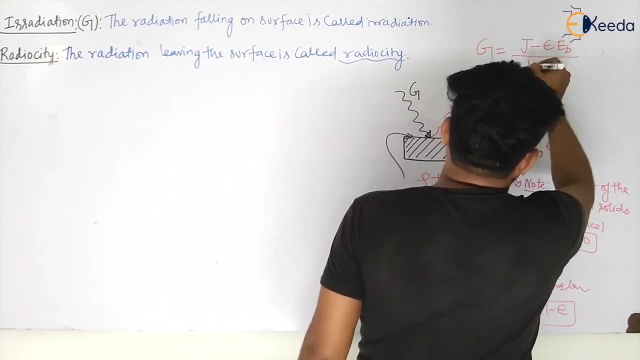 is equal to. we have calculated the value of G, I think. so this is nothing but what, J minus epsilon E into E, b divided by 1 minus E. so that was your equation 1,. okay now so my. 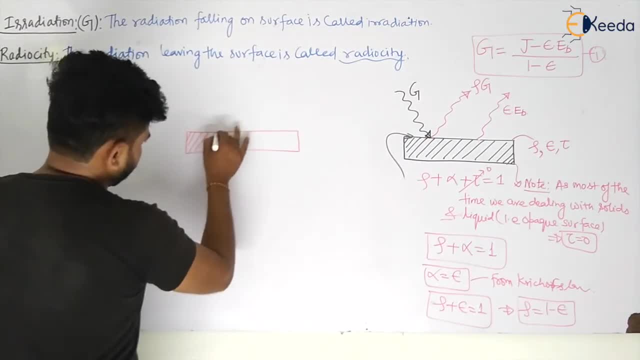 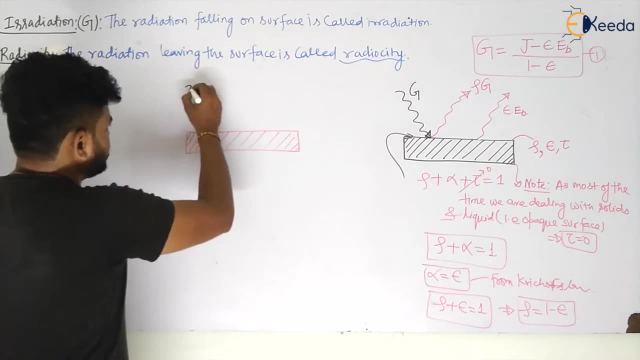 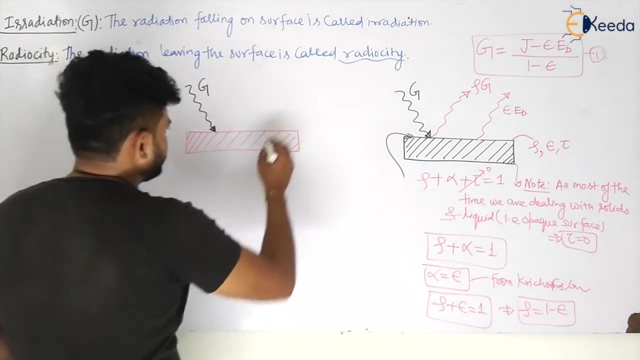 dear students, if I am having this surface, let us say I am having this surface- this is absorbing some radiation. so some radiation is coming to this- that is your G, and some radiation is leaving this surface. my dear students, some radiation is leaving this surface. 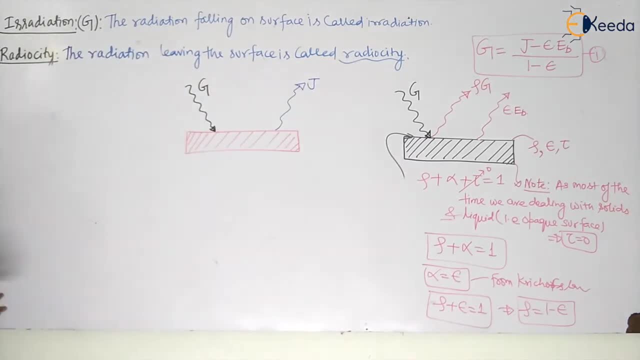 let us take J, that will be J. okay now the net radiation exchange with the surface. net radiation exchange with the surface is equal to. Q is equal to. let us say Q is equal to, that will be nothing but J. that is the radiation leaving the surface, and radiation. 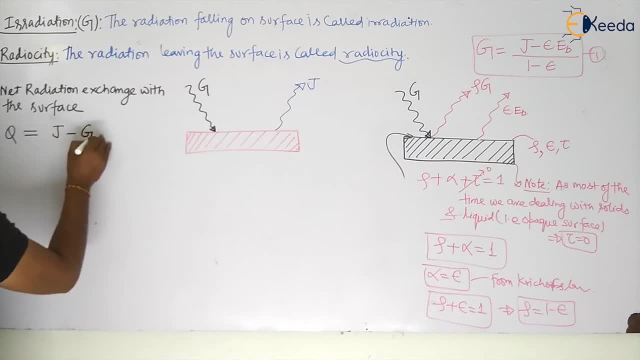 coming to the surface. so this will be j minus g. okay, so let us put the value from g from equation number one. this will become j minus j minus e, of ev divided by one minus e. so let us take that lcm of this. this will become one minus e, and i have to multiply this equation with this, so this: 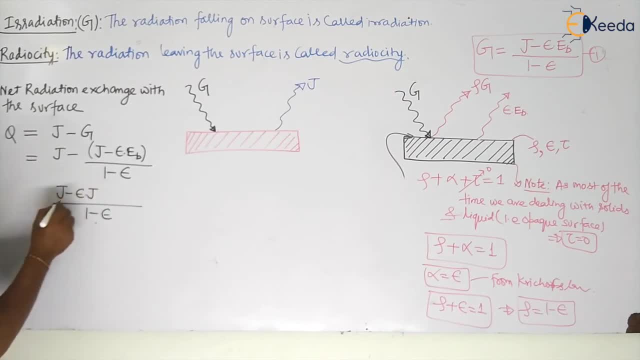 will become j minus e of j, e of j. okay, then i have to take that minus inside, so this will become j minus again. this will become e of ev, e of ev, my dear students. so j and j will go. so i will be left with only e of ev minus e of j, divided by one minus e, my dear students. so this will become. 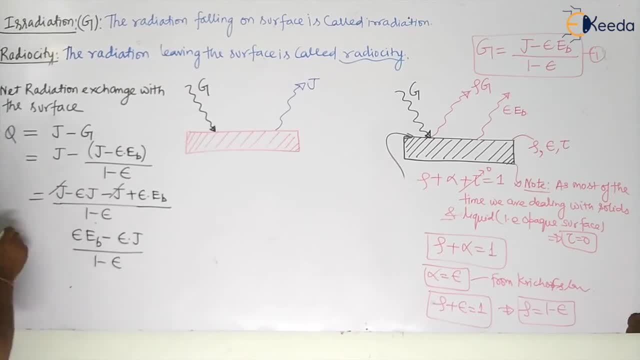 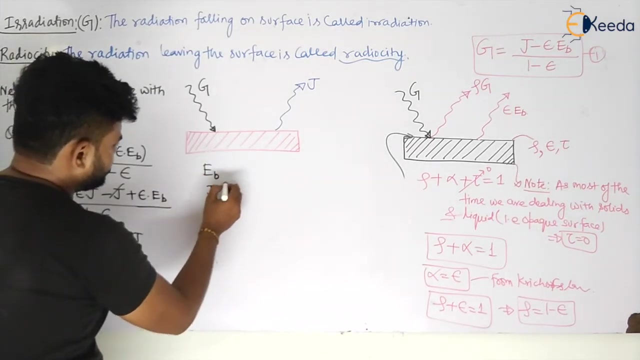 if i will take e out, so this will become that implies q is equal to q is equal to e. i am taking out this will become eb minus j and 1 minus e minus students. eb minus j and 1 minus e minus my students. now if, if i am taking this, these both terms like eb and j to be total, to be total, 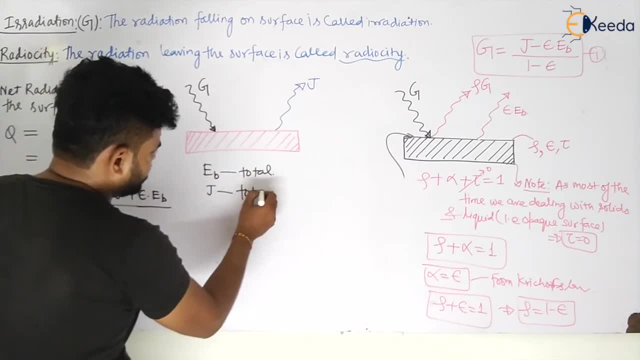 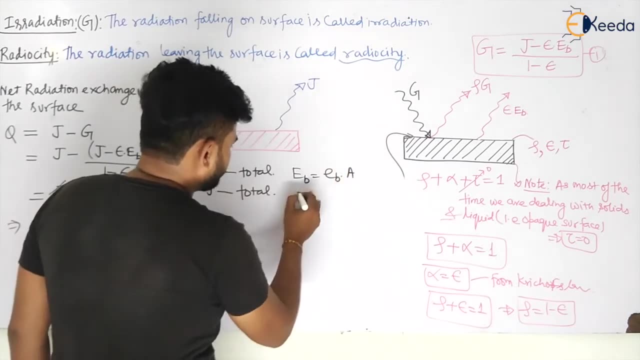 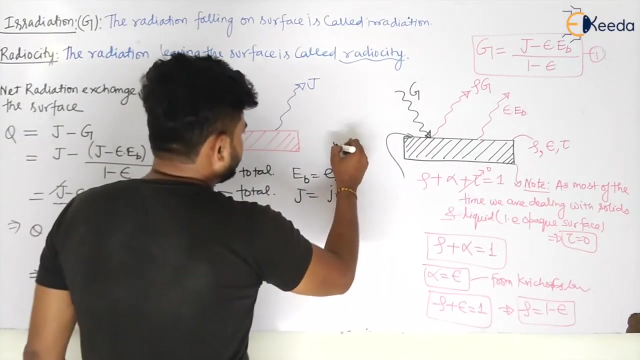 total, not per unit area. i am taking to be total. so can i take this like this: so eb can be written as a small eb dot area and j can be written as a small j into area, my dear students, so can i put like this: if this is per unit area, that is what per meter square, this is also what per meter square. 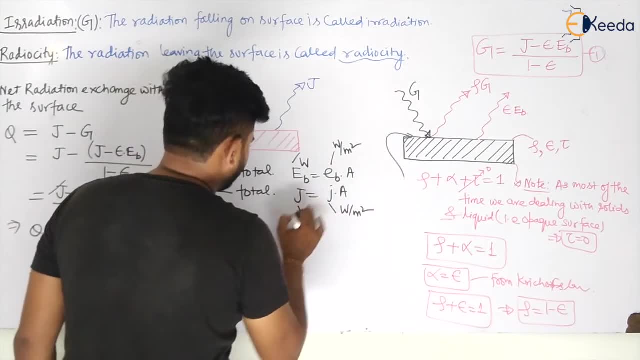 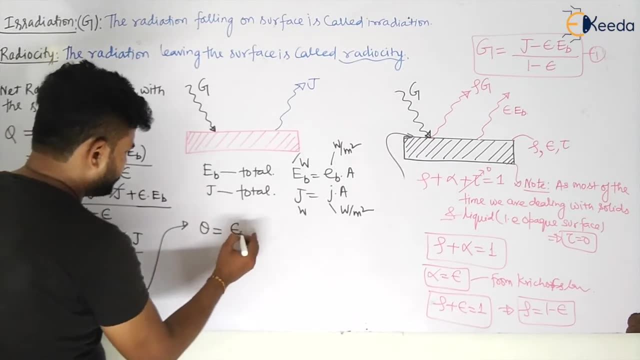 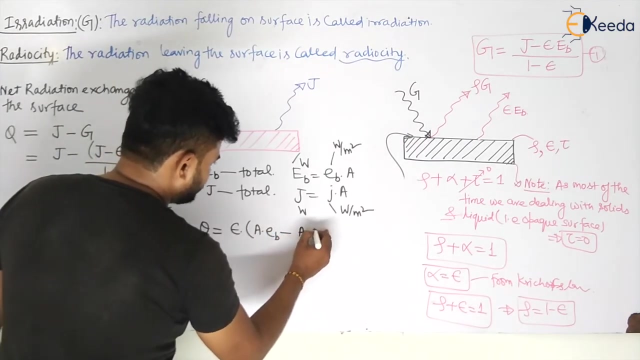 my dear students. so this is what the totaling this was in totaling what? so? let us take it so, putting the value of these equations, what i will have this will become: q is equal to e dot eb, which is now area- into eb- small eb per unit area, minus area- into j, small j, my dear. 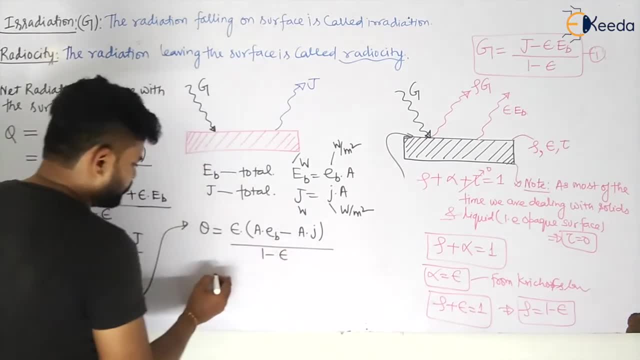 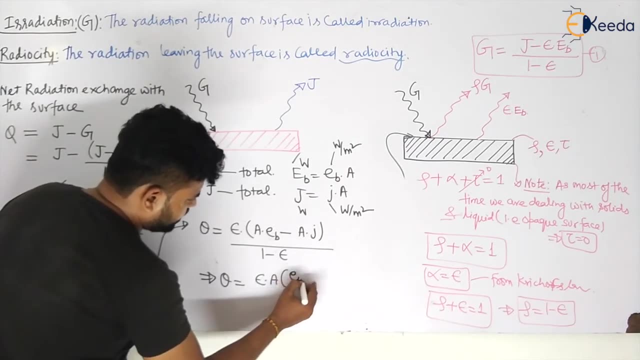 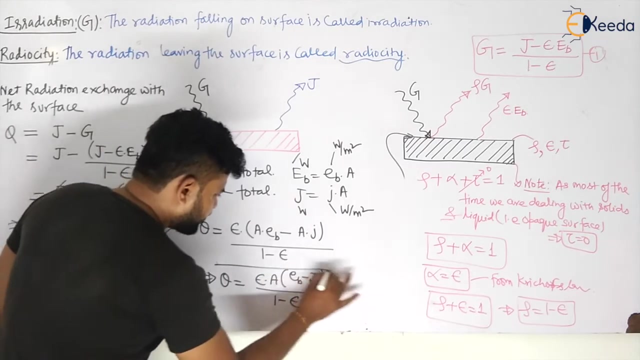 students. so this will take the form 1 minus e. so this will become equal to. q is equal to e and area i am taking out this will become eb minus j. my dear students, eb minus j divided by 1 minus e. so can i have the analoging of this? 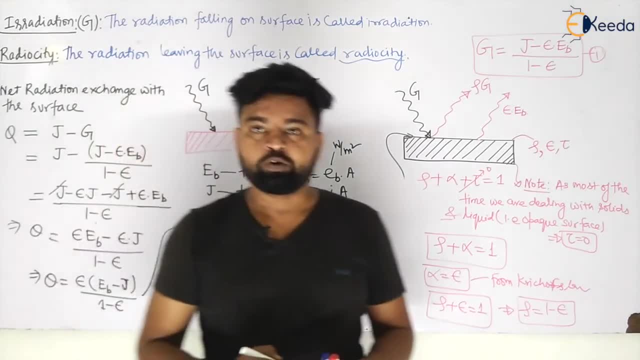 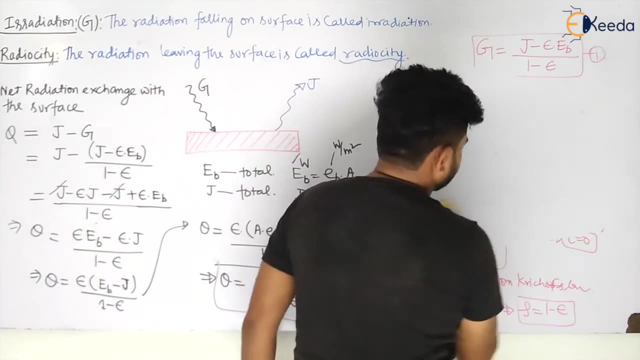 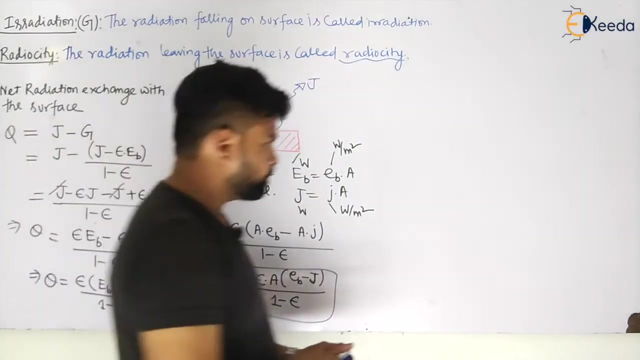 with something like called ohm's law, or we have seen in the conduction that electrical analogy. let us see so for this surface, my dear students, what it will become. let us see now, i am having one surface only. let us say i am having only one surface. i will take a different. 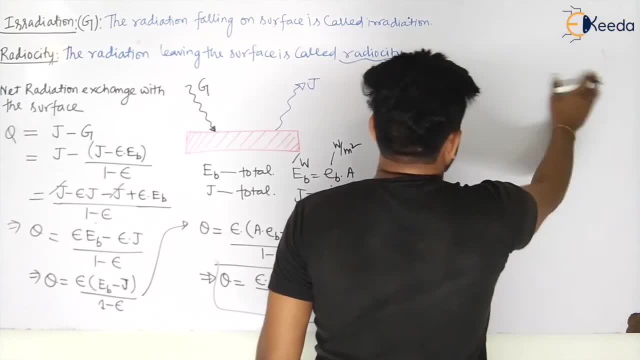 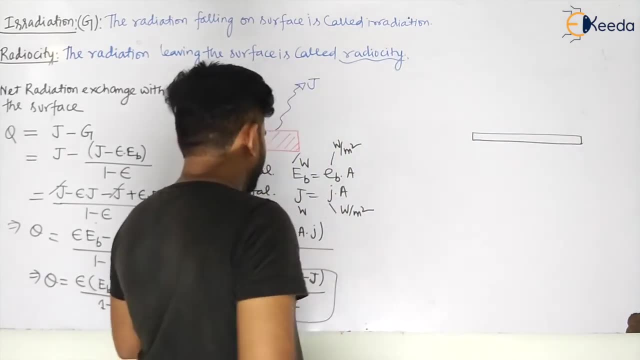 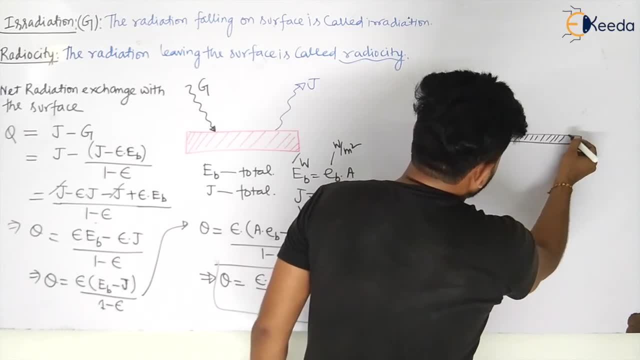 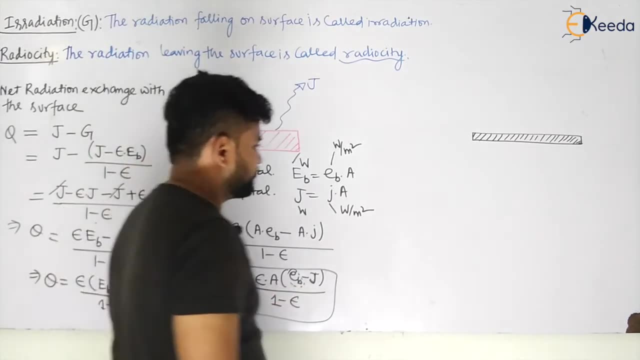 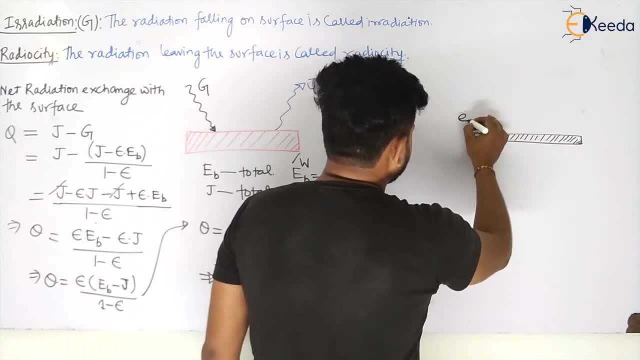 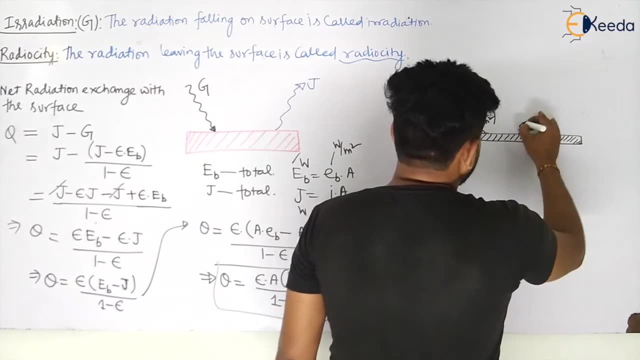 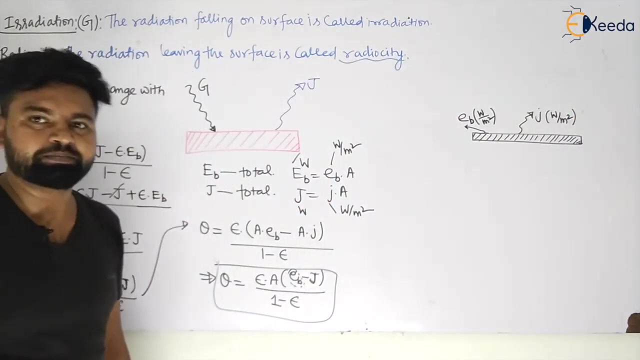 this is nothing but like if eb is there, that is, it is emitting radiation per unit area watt per meter square, and also this is leaving the total radiation j small j per unit area watt per meter square material, which is also leaving some radiation watt per meter square. so in between, 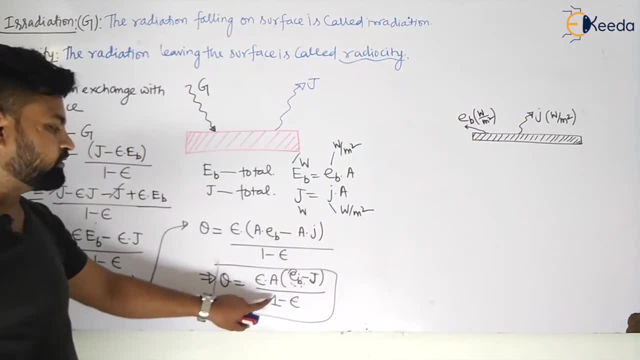 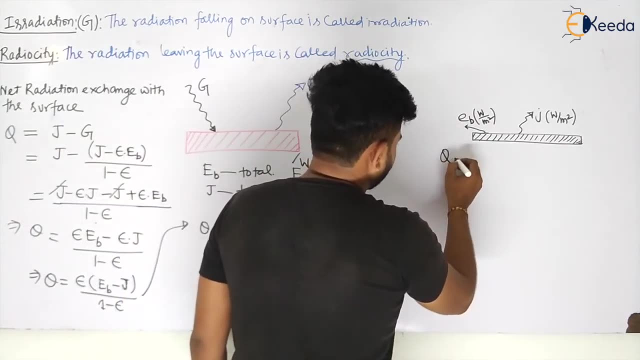 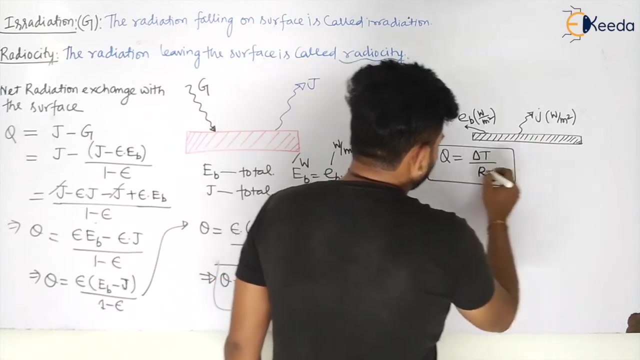 eb and j. there is some resistance. that is what? what? nothing but one minus e into ea. let us take it in the form of this: so you know that q is nothing but equal to delta t by r. thermal media students are thermal. you know this equation very well, but you also know that i is equal to. 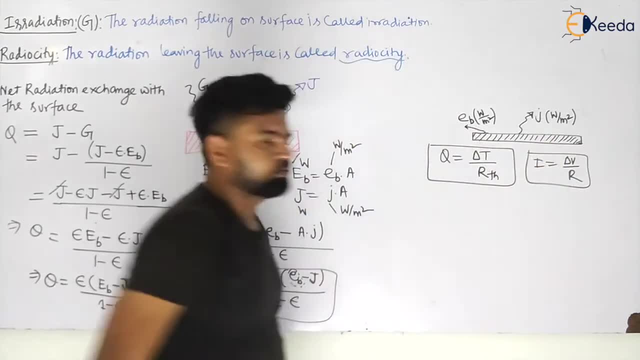 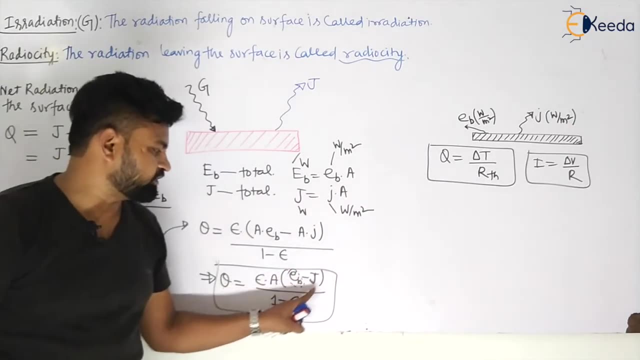 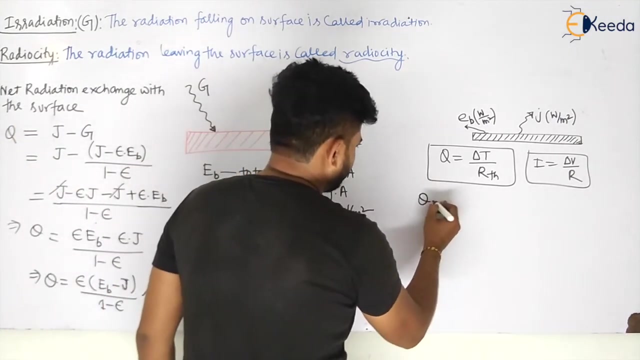 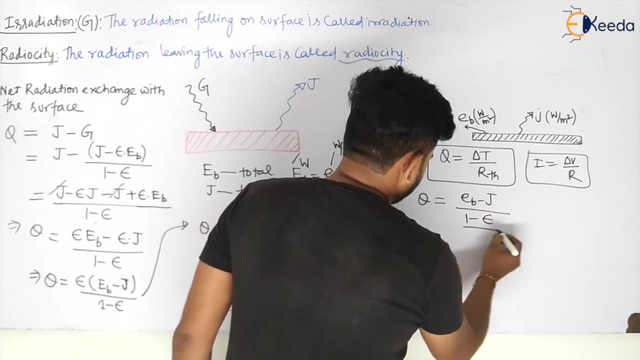 delta v by r. now we know this equation, also these two equations. you know if i will compare these both equations and i will assume that it is a potential difference for radiation heat exchange, radiation heat exchange. so can i calculate the resistance? yes, so it will. it will become equal to q into eb minus j, divided by one minus e upon ea media. 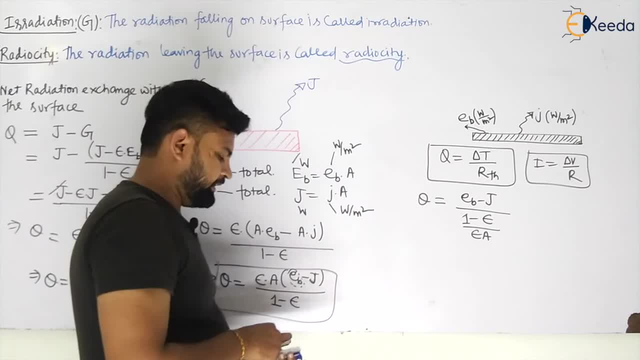 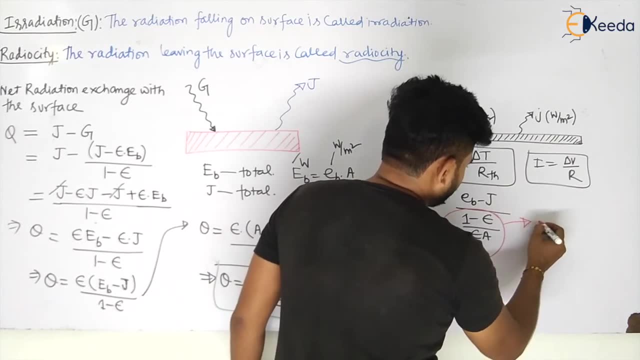 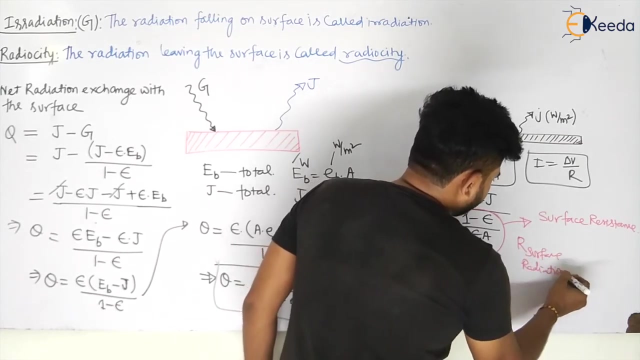 students, where one minus e upon ea will be your radiation resistance for this particular surface. that will be your surface, that will be called your surface resistance, my dear students. so one minus, that is our surface for radiation, for radiation will be equal to one minus e upon e a. so 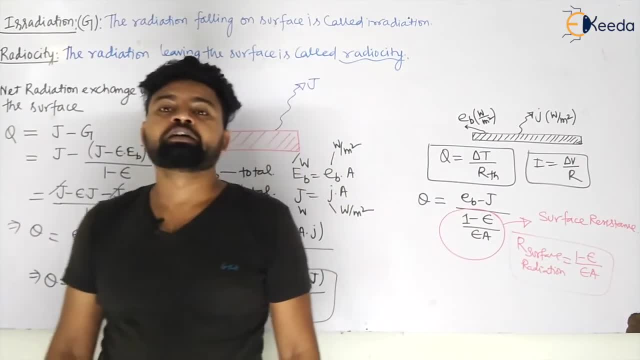 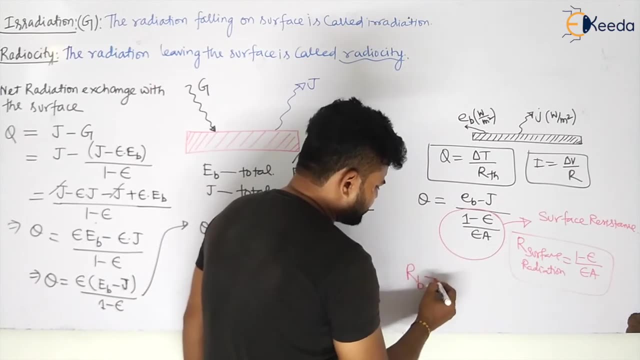 for this surface. that emissivity is defining the surface. resistance, my dear students, why does c if it is a black body? can i calculate the resistance for the black body? that is one minus zero or one minus what is the emissivity for black bodies? or eb is equal to one, and we know. 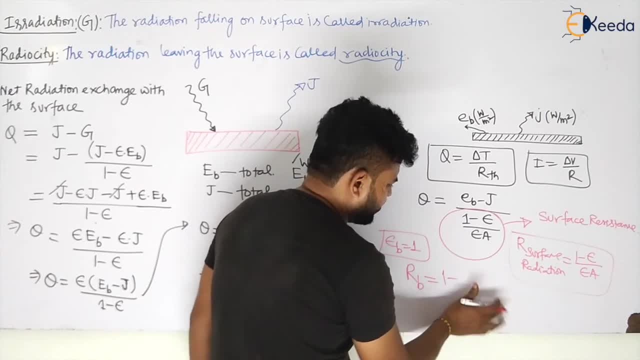 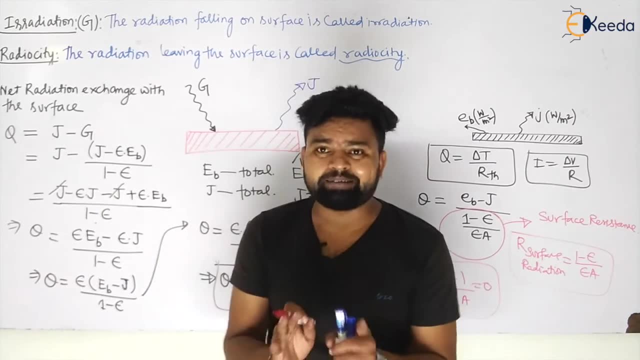 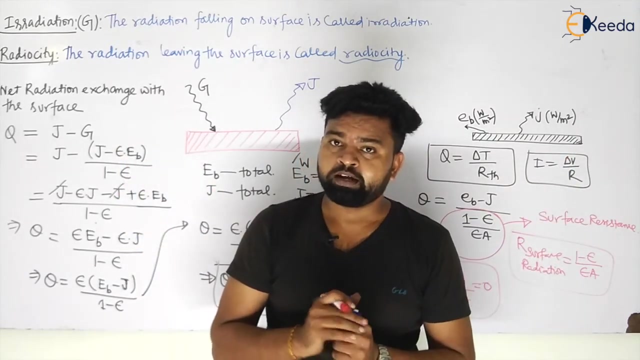 so rb will become equal to one minus eb, that is equal to one divided by one into a. so this will become zero. oh my god, for the black body, the surface resistance is zero. that's why it is emitting the maximum radiation, okay. and as the emissivity is increasing, 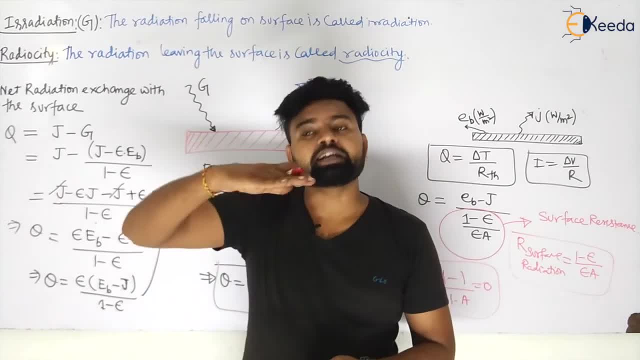 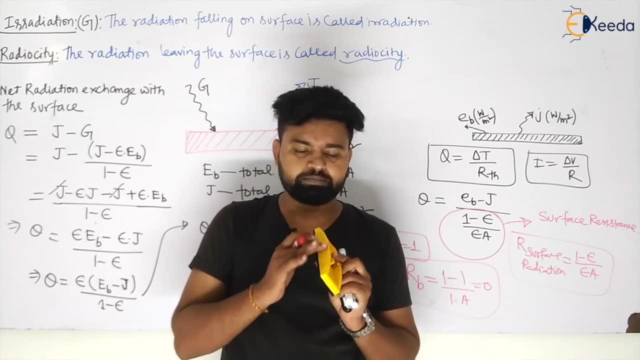 the resistance, that is, surface resistance of the body, is increasing. my day of students. let us say: if this is your surface and your half it is, that that is emissivity. if there is emissivity, or this particular surface, from zero to one, if it is increasing, then 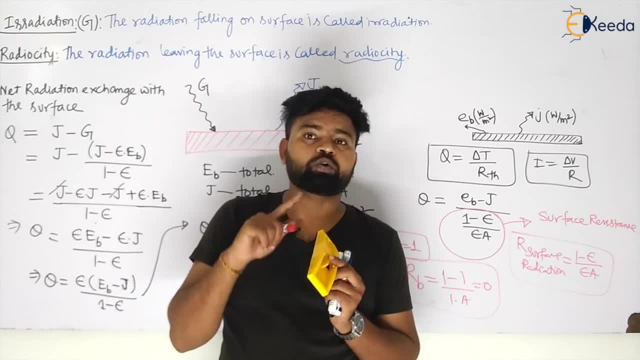 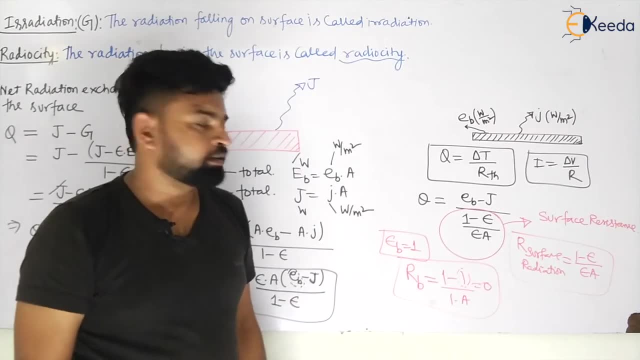 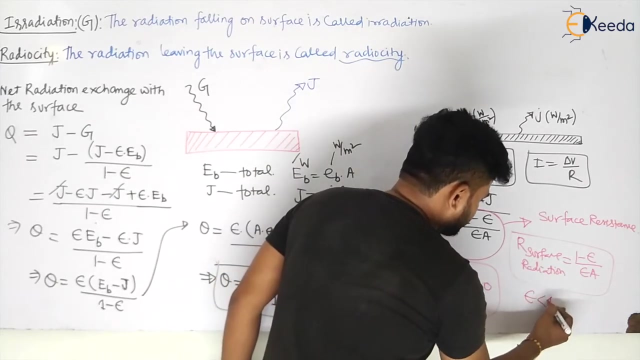 resistance is increasing. but if the emissivity is equal to one, if the emissivity is becoming equal to one, my dear students, then the resistance is what? the resistance is equal to zero. But if the emissivity is less than 1,, my dear students, then this will have some surface resistance, my dear students. 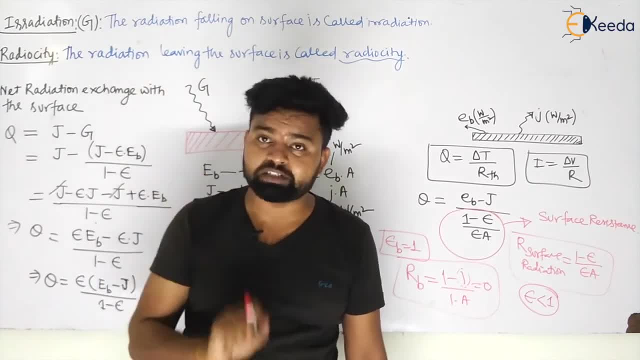 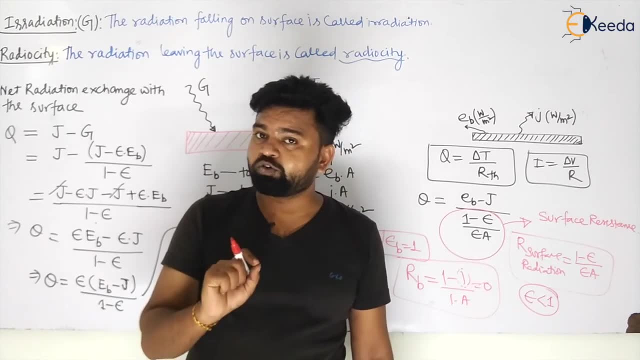 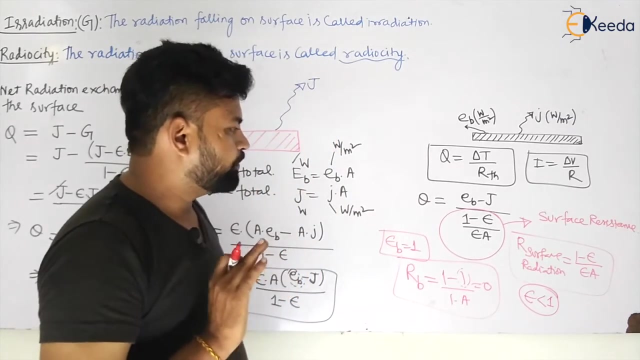 So every non-black surface which is having some emissivity will have the surface resistance. okay, Only the black body which is having emissivity equal to 1 will have the surface resistance equal to 0, okay, Now hope you have understood the concept. 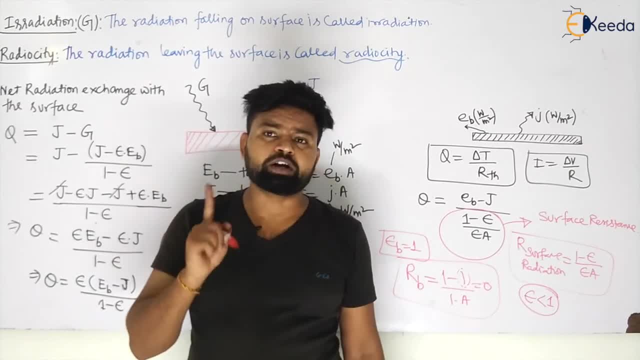 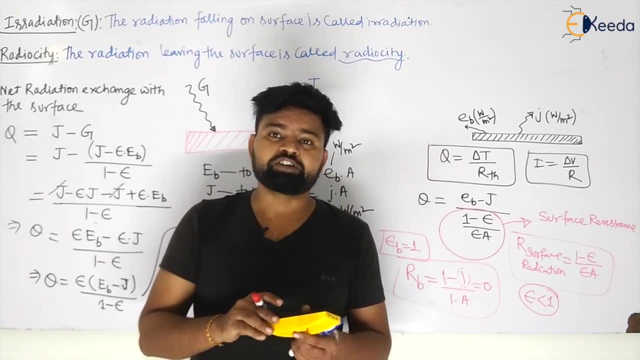 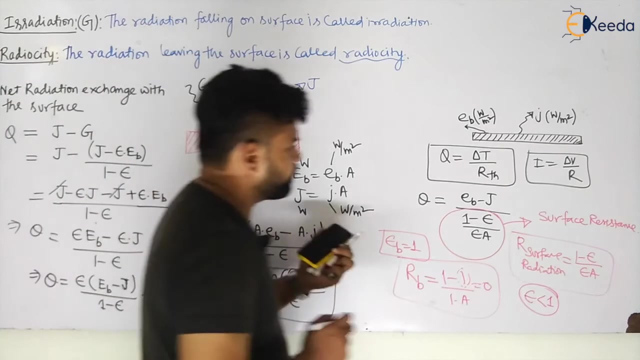 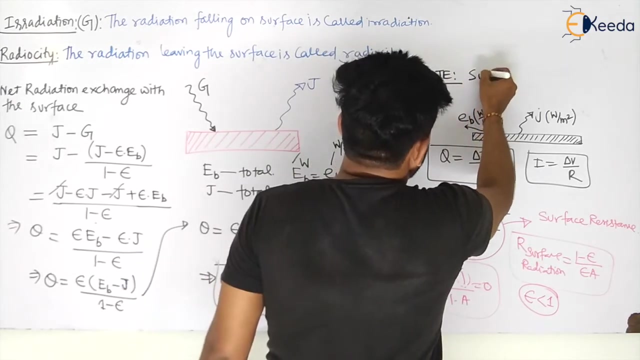 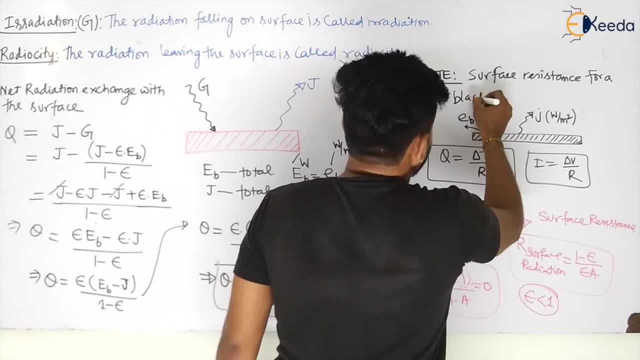 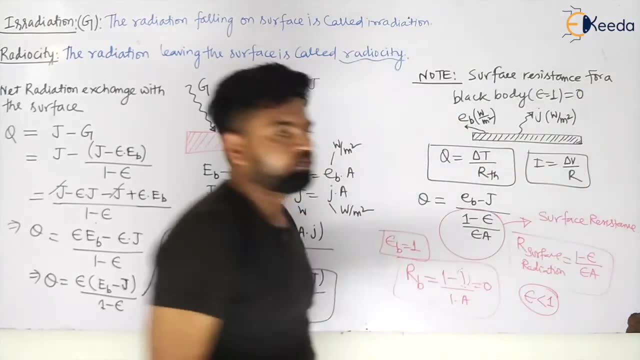 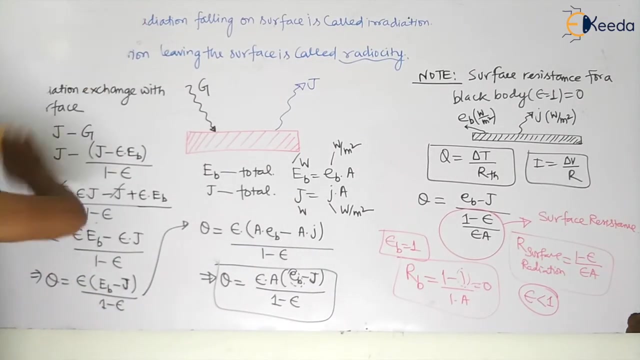 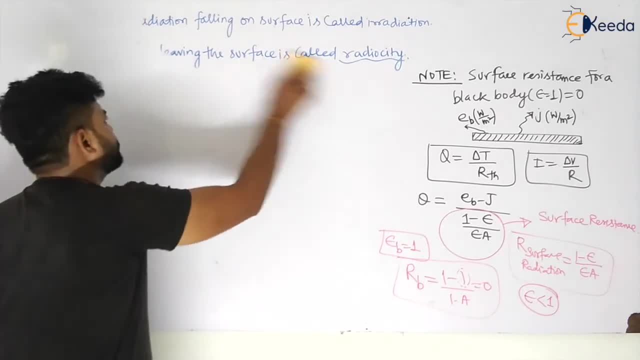 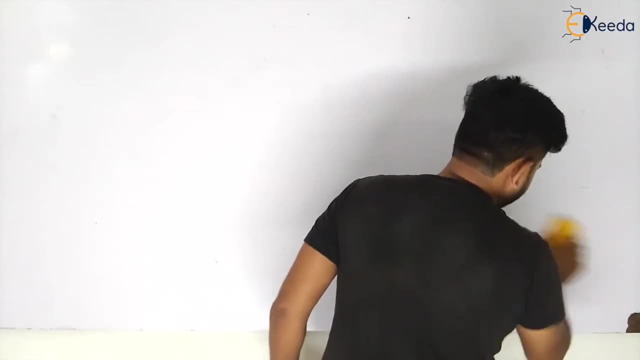 This is the most important for your grade. So just focus on the goal. my dear students, I hope you are feeling the concept now. Let us feel it More carefully. Let us feel it more carefully. Let us see, my dear students, 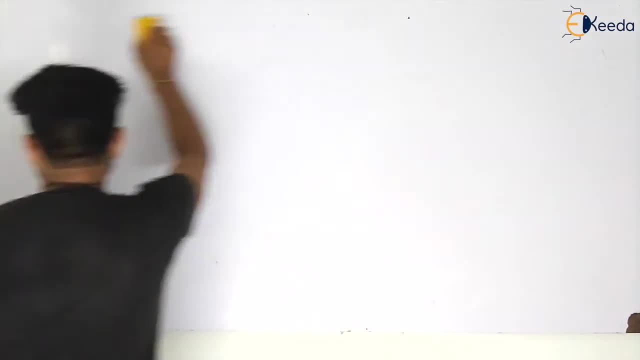 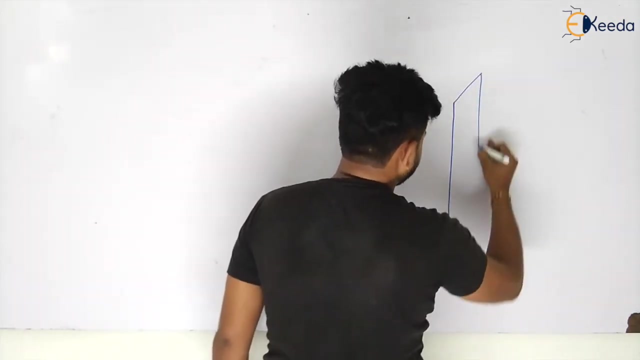 Let us see Now. let us see If I am having the two surfaces. if I am having two surfaces, let us take two surfaces. my dear students, If I am having two surfaces, this is again your surface 1.. Let us take surface 1.. 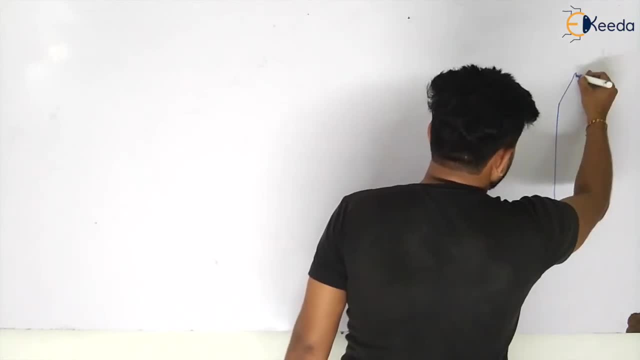 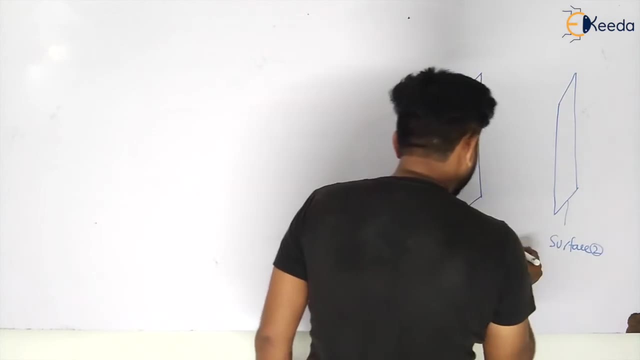 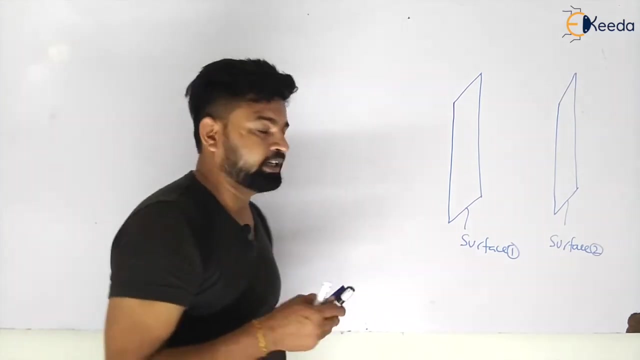 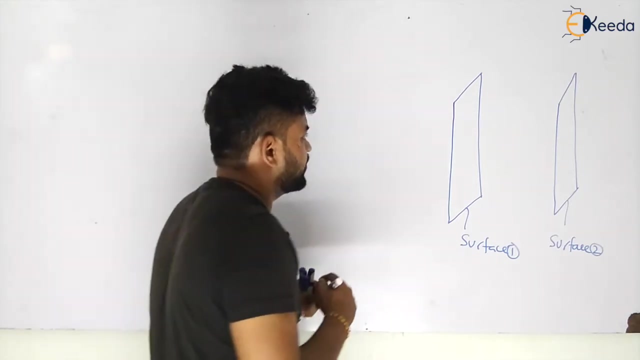 And again I am taking the surface 2.. So, my dear students, this surface 1 will have some potential difference because of for what? for radiation I am talking. So just feel the analogy, so that you will be building all the concept in your mind. you don't have to remember anything, just learn here. okay, let us see. 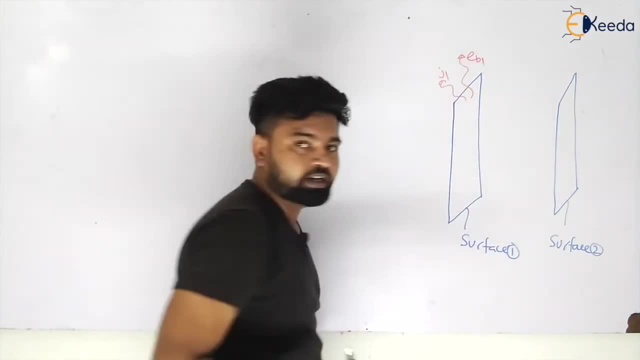 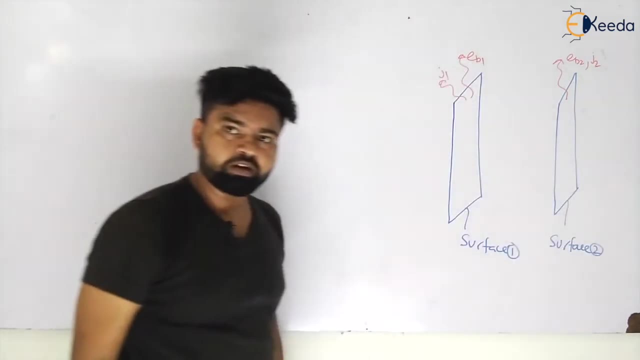 This will be having some radius of the J1, my dear students- piont area, all these things. Similarly, this surface is having EV2.. And some J2, my dear students. Okay, Now this surface is having some resistances. 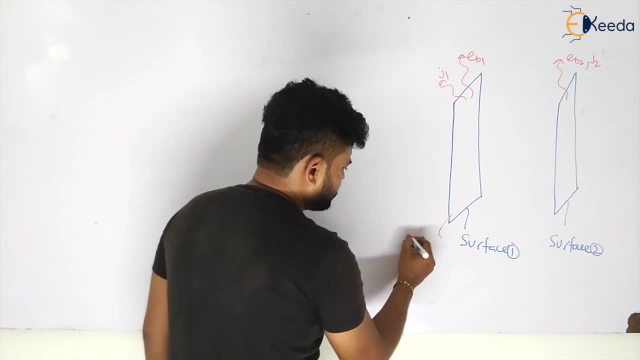 This surface is having some resistances, which is nothing but what. That is our surface. 1 will be equal to 1 minus. That will be 1 minus. Let us take: E1 is the emissivity of this and E2 is the emissivity of this surface. my dear students, 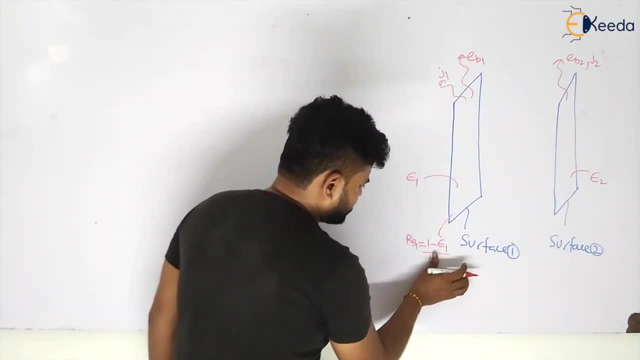 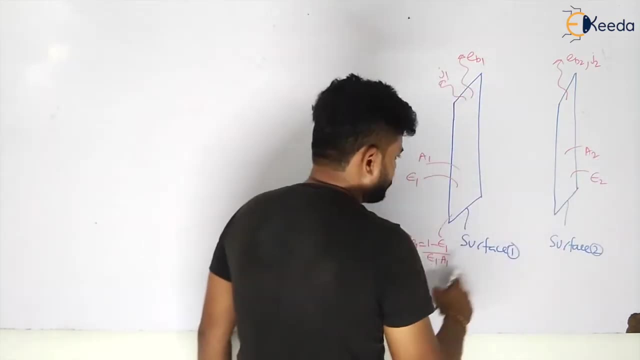 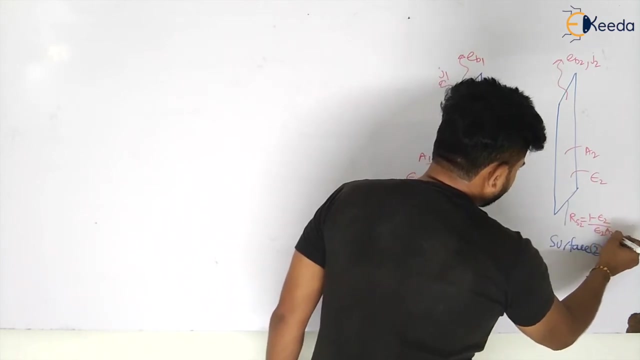 So this will become 1 minus E1 upon 1 minus E1 upon E1A, A1.. Okay, E1A1.. Now, similarly, for this surface, what will be the surface resistance to This? will be 1 minus E2 upon E2A2,, my dear students, E2A2.. 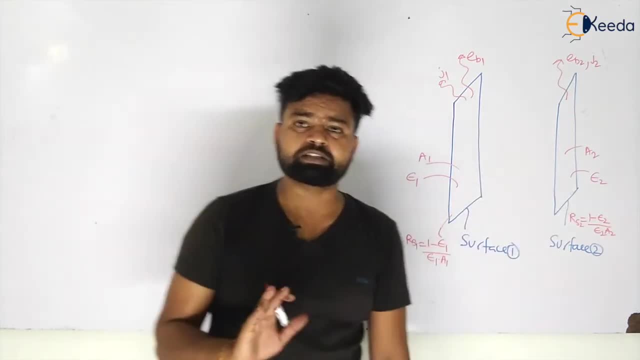 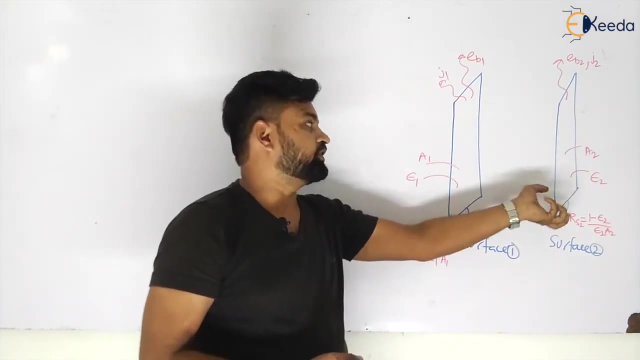 So now that these particular surfaces are having some resistances, So so when the radiation is coming out from this maybe falling on 2, and the radiation which is coming out from 2 may be falling on 1.. 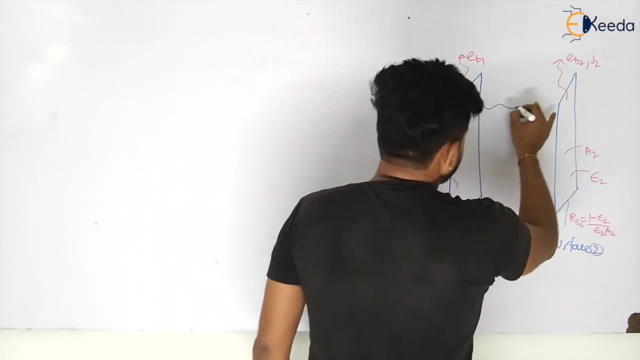 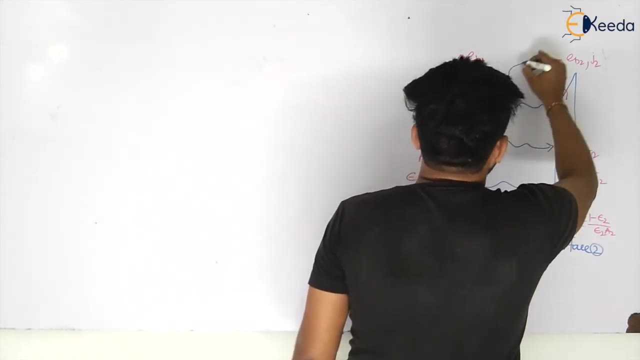 So what it will become, Let us see. So some radiation is coming out from this and falling on 2. And that fraction of radiation will be called your shear factor, my dear students, And some may be going out in all directions. 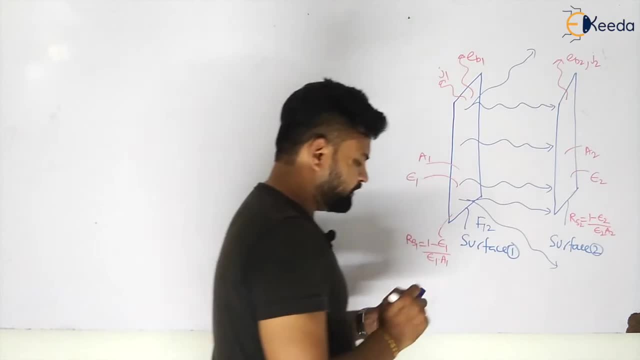 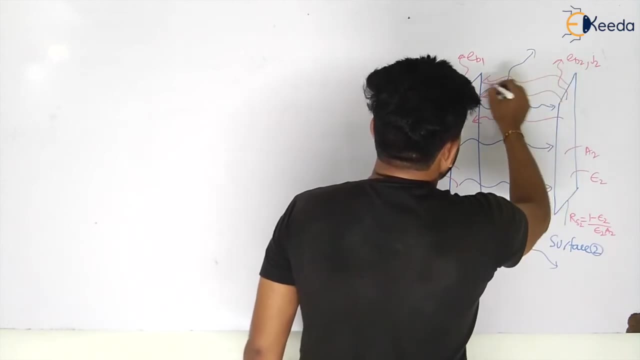 So what will be this? This will be F1,, 2,. my dear students, Similarly, some radiation is coming out from 2 and falling on 1.. Yes or no? Now, this is falling on 1, and some may be coming out in these directions. 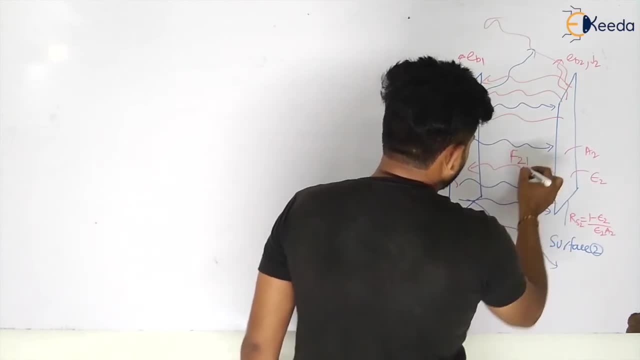 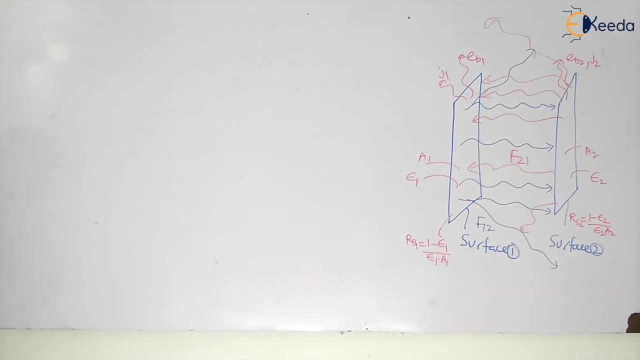 Yes or no? Yes, And this will be called your F2, 1,, my dear students, F2, 1.. So let us calculate this. Let us calculate this Now. Now let us see. Let us see: the total radiation leaving the first surface is what? 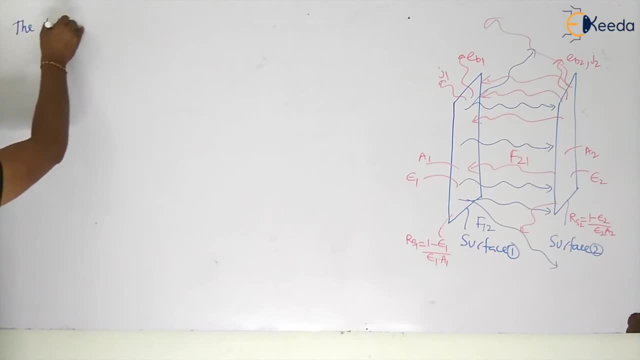 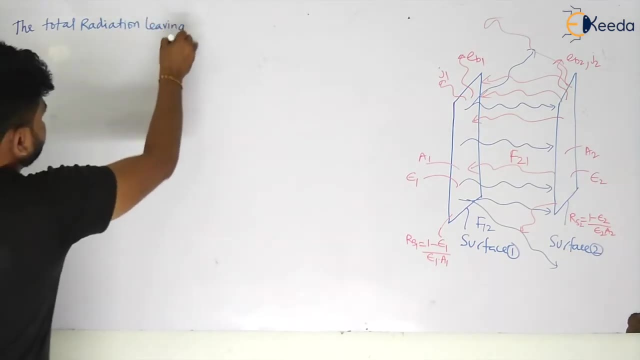 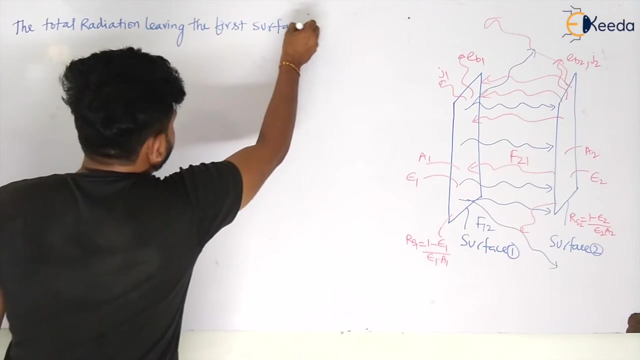 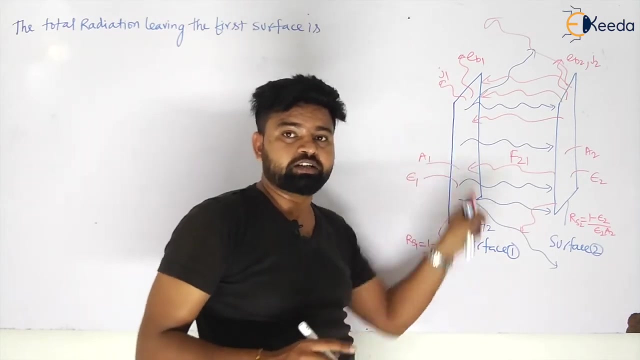 The total radiation, radiation leaving the first surface surface is: So what was the radiation which was leaving 2? So leaving 1, it was J1. only That was your radiosity. radiosity, the total radiation coming out from the surface 1.. 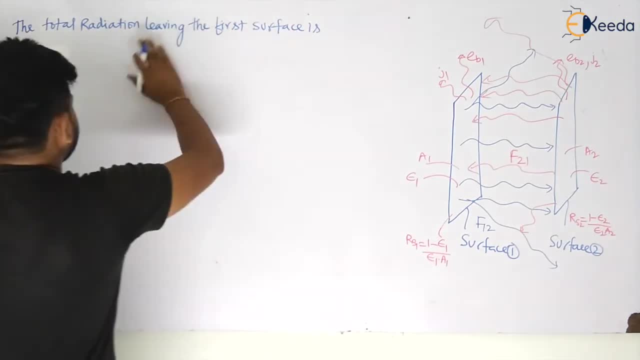 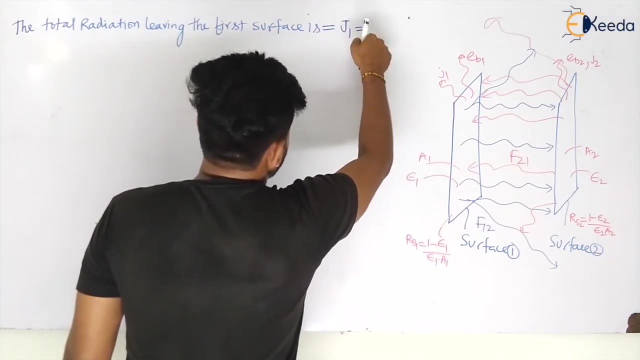 That was your radiation, that was your J1.. The total radiation leaving the first surface is your J1,, my dear students, J1.. And this can be taken as small j1 into A1.. Yes or no? Small j1 into A1. 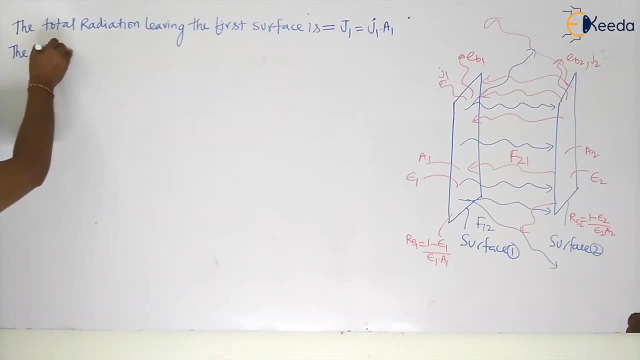 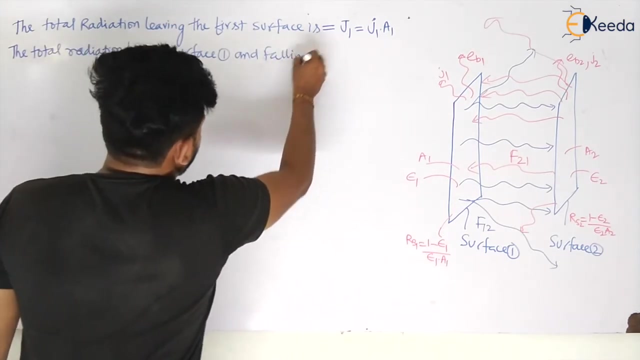 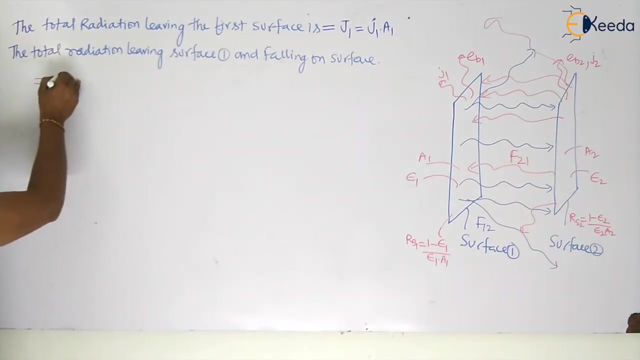 Now, the total radiation which is coming, leaving surface 1 and falling on 2, the total radiation Leaving surface 1 and falling on surface 2, on surface 2, will be equal to what, my dear students? This will be nothing but equal to J1, A1. 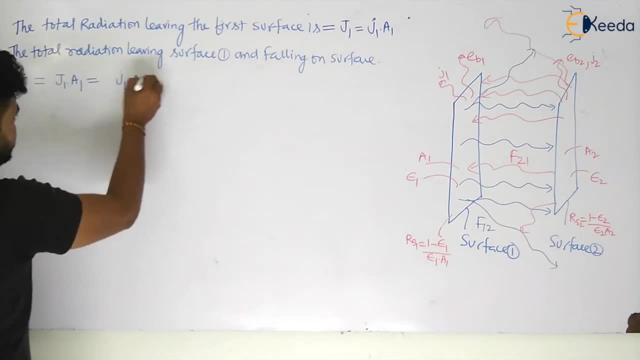 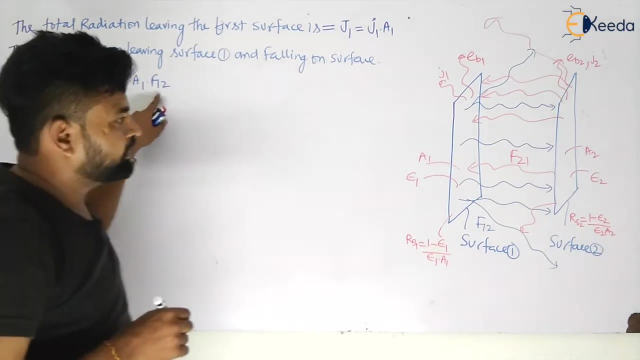 Or I can write like small j1 into A1, into that will be F1, 2,, my dear students, into F1, 2.. So that is fraction of radiation. So F1 will decide that how much radiation. 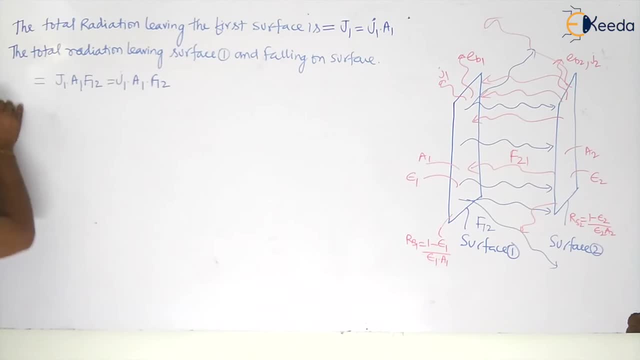 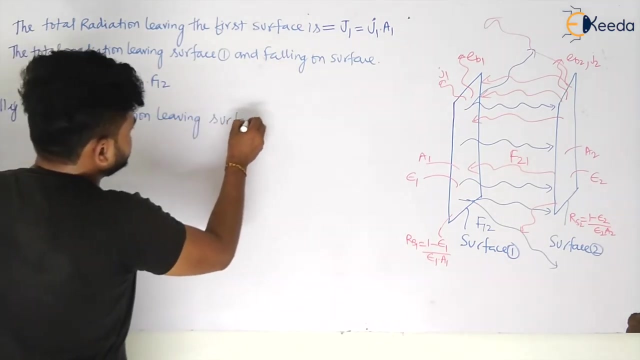 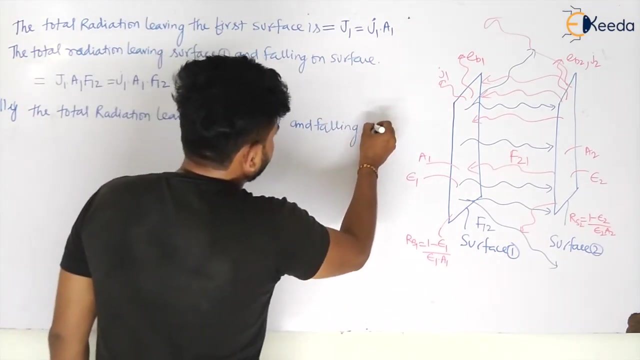 Radiation is leaving that and reaching on the 2,, my dear students, Similarly, similarly, we can know the total radiation, the total radiation leaving surface 2, leaving surface 2 and falling on surface 1, falling on surface 1, my dear students. 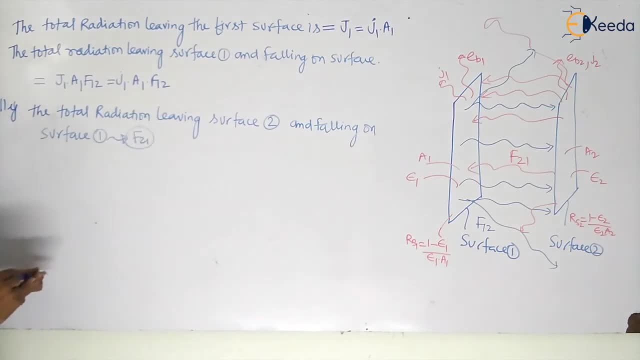 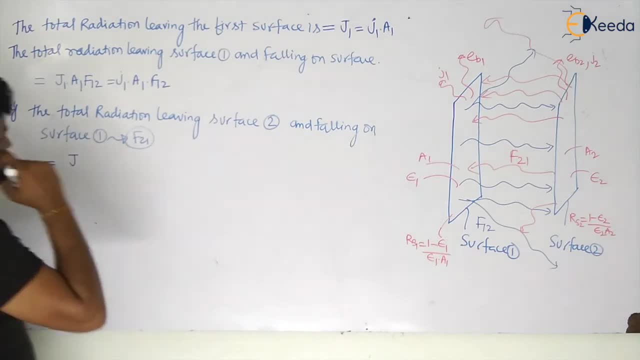 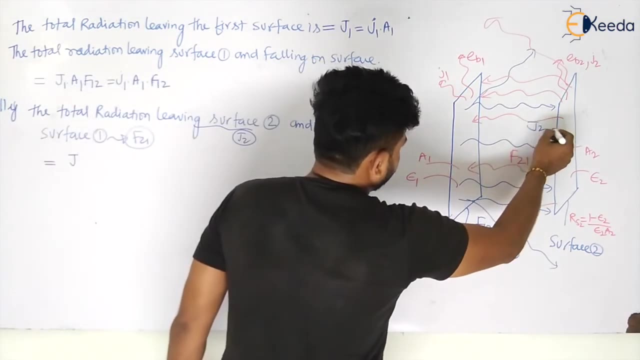 So this will be equal to nothing but your and total radiation leaving the surface is nothing but your J2.. Leaving the surface, 2 is J2.. So this you can take J2.. This you can take J1,. my dear students, 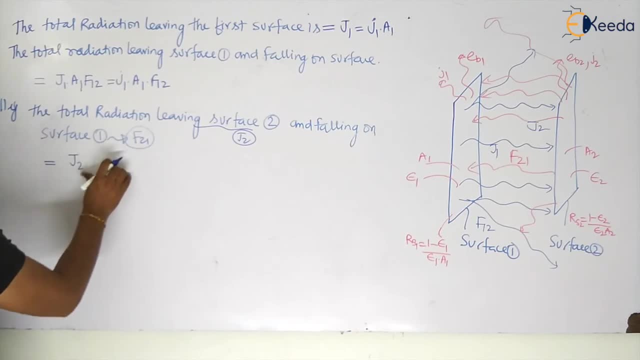 So this will become J2 into J2, into F2, 1.. Or, if you are taking per unit area, if this is your total, so you can write this: J is small, J2 into A2, into F of 2, 1,, my dear students, F of 2, 1.. 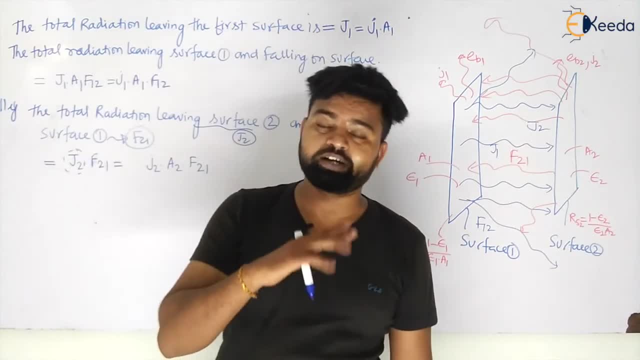 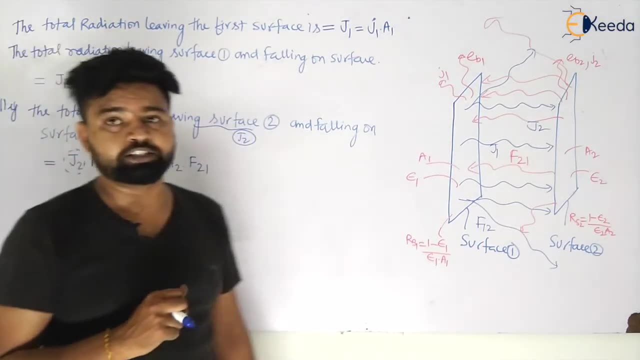 So that is the total radiation which is leaving the surface 2 and reaching to the surface 1.. So can we calculate the net radiation exchange between two bodies? Yes, we can calculate the net radiation exchange. Let us see. Let us see, my dear students. 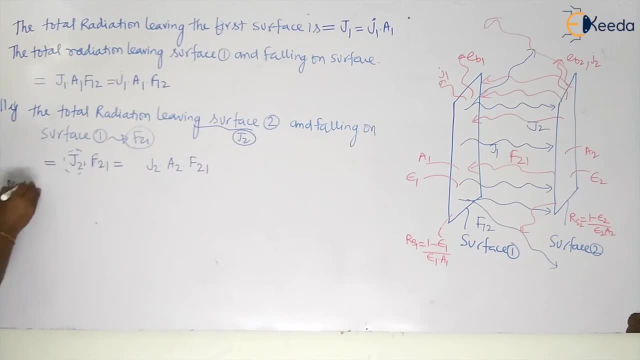 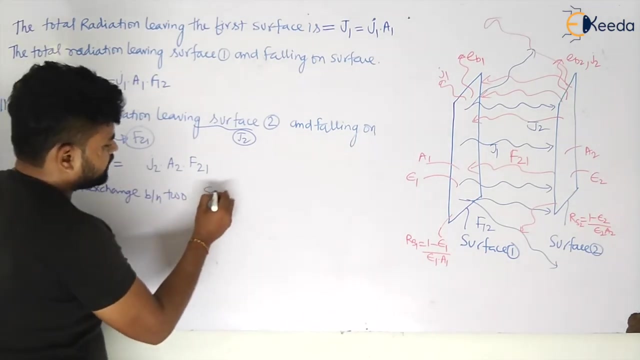 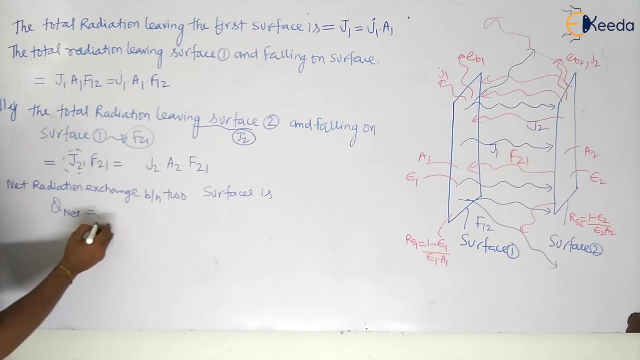 So the net radiation exchange between two bodies, net radiation exchange, Let us see So. the net radiation exchange between two bodies will be given as, or we should say, surfaces. Two surfaces is, let us take Q. net is equal to nothing. but that will be your small J1,. 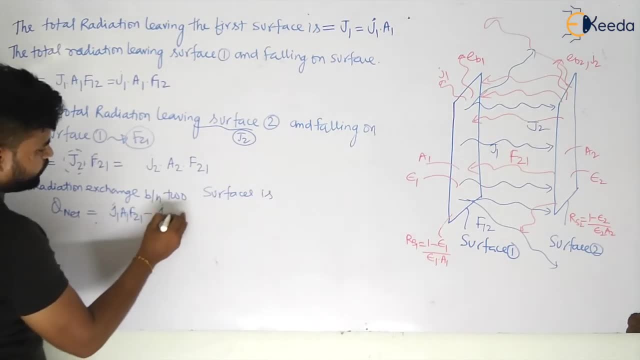 A1,, F1, 2, minus small J2, A2, F2, 1.. Yes so, my dear students, so this will become nothing, but I can take A1, F2, 1, A2, F2,. 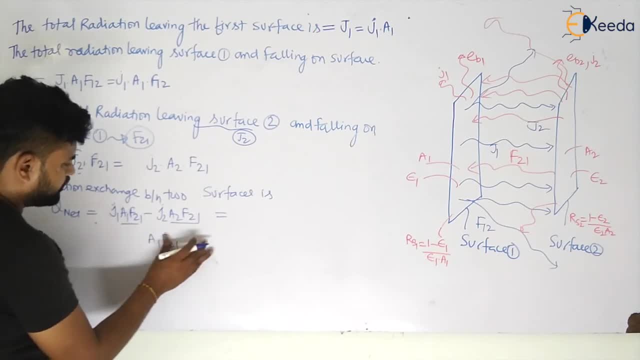 1.. So this will become nothing, but I can take A1, F2, 1, A2, F2, 1.. Why I will use the reciprocity theorem. This will have to be A1, F1, 2.. 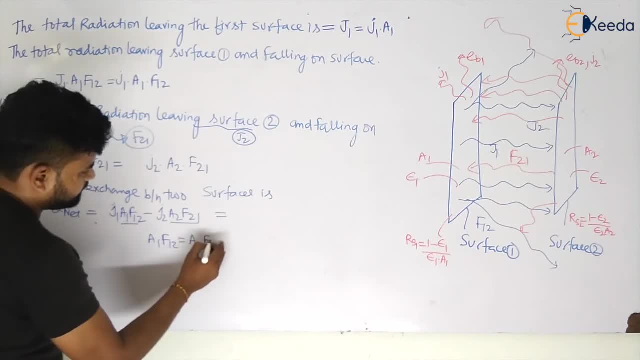 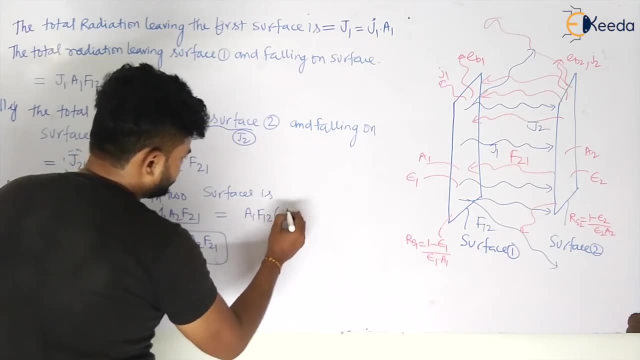 A1, F1, 2 is equal to A2, F2, 1 from reciprocity theorem. So I can directly write like A1, F1, 2 into small J1 minus small J2,. my dear students, 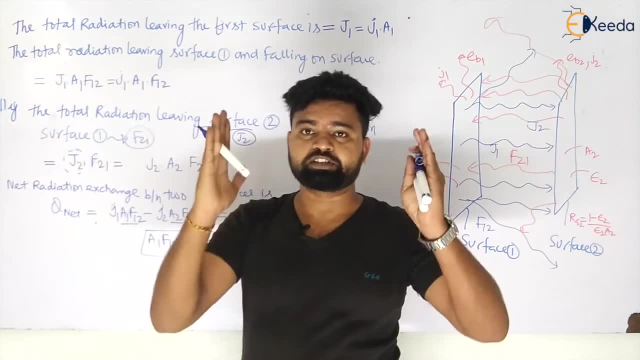 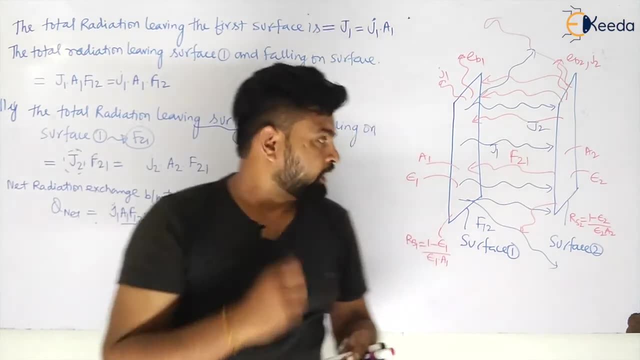 So this will be the net radiation: heat exchange between the two surfaces because of the orientation or geometry. my dear students, Now let us see. let us see, this is the net radiation. Now, if this is leaving some radiation, this is also leaving some radiation, some radiocity. 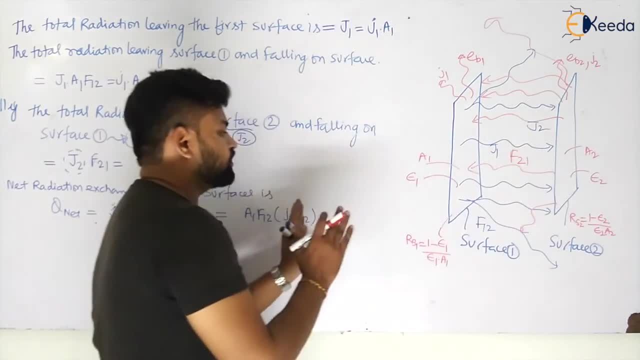 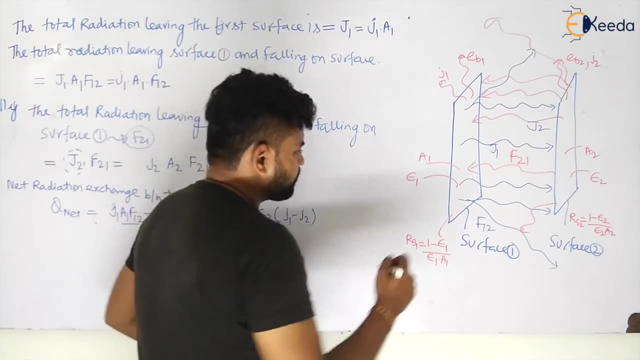 is having this surface, some radiocity is having this surface and, because of this, there is some heat transfer between those surfaces because of radiation heat exchange. Now let us see if this is having your J1,, my dear students, and this is having your. 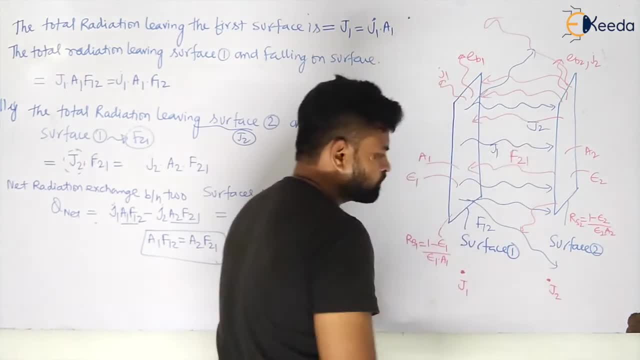 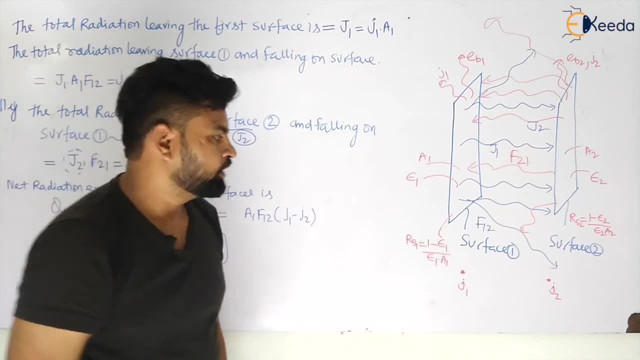 J2,. this is having your J2,. let us take it as small: J1 and J2 per unit area. okay, J1 and J2,. my dear students, So there is some net radiation heat exchange, Can I assume, or can I compare this with a potential difference? 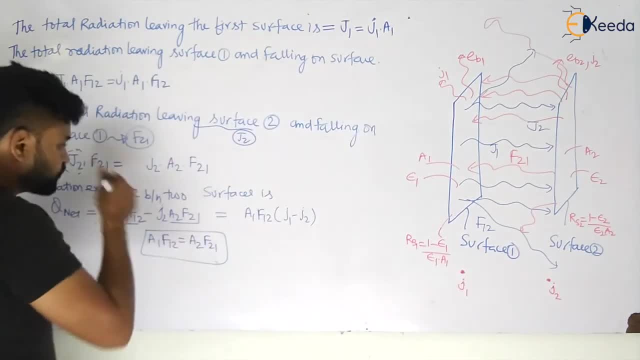 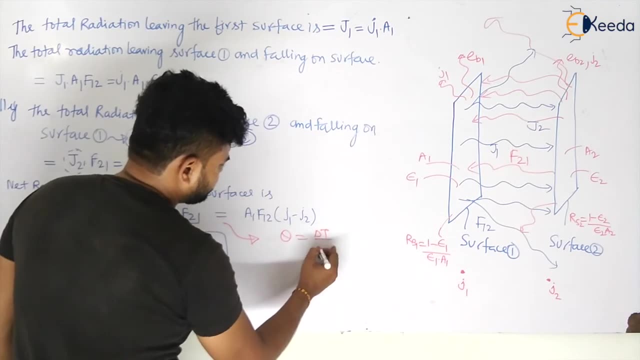 Yes, because it is having also some resistance. So if I will compare with, like our conduction equation, as you have seen that Q is given by delta T, by R thermal, my dear students. So now delta T- I am taking this value, and Q- we have already this, so Q net will be. 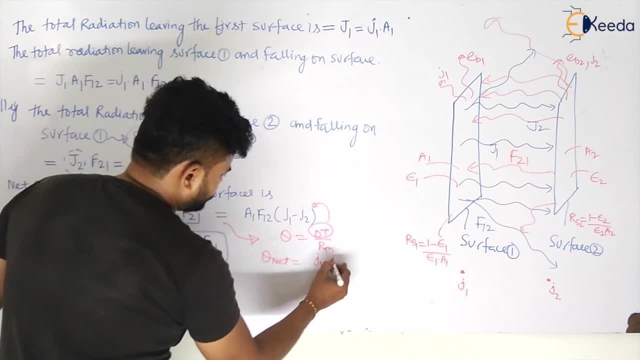 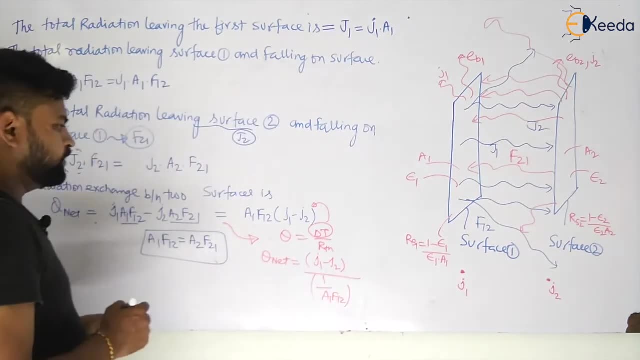 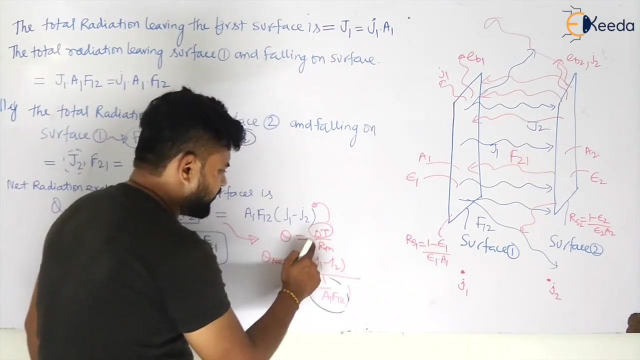 equal to nothing, but equal to, That is small J1 minus J2 divided by 1, by A1, F1, 2.. So in this case, if I will compare with this equation, then this value, my dear students, this value will be equal to your R resistance, and this is called your. that will be some. 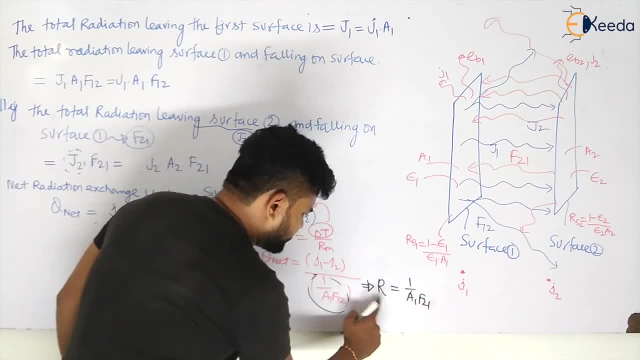 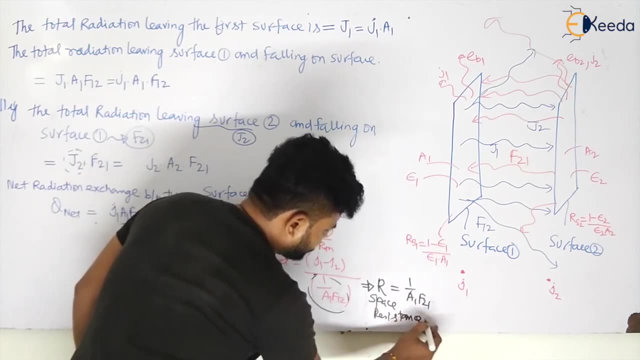 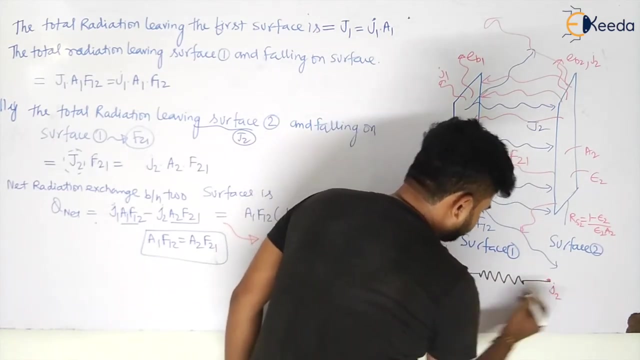 R, which is nothing but 1, upon A1, F1, 2, and this is called your space resistance, my dear students. So between these two bodies, these two surfaces, there will be some space resistance. that will be nothing but A1, F1, 2, that will be equal to this much, my dear students, and 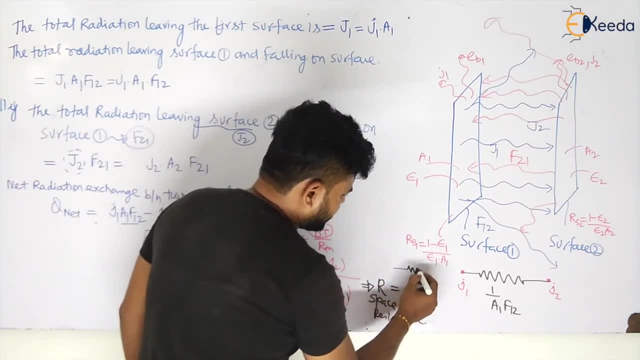 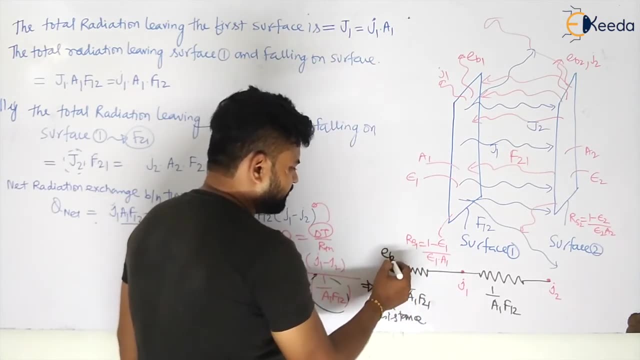 also, we are having R S1,. yes, we are having R S1,. my dear students, we are having also that surface resistance, one surface resistance between what that is nothing but A, B and this. also, we are having that surface resistance too. 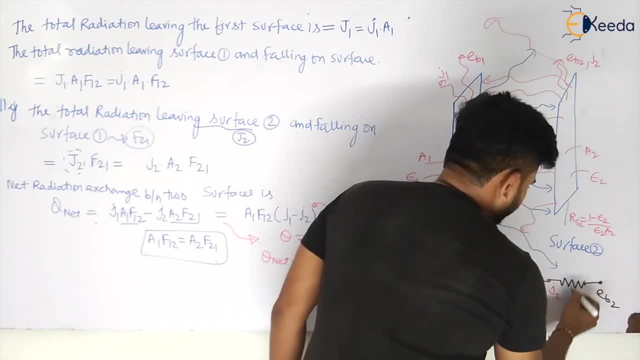 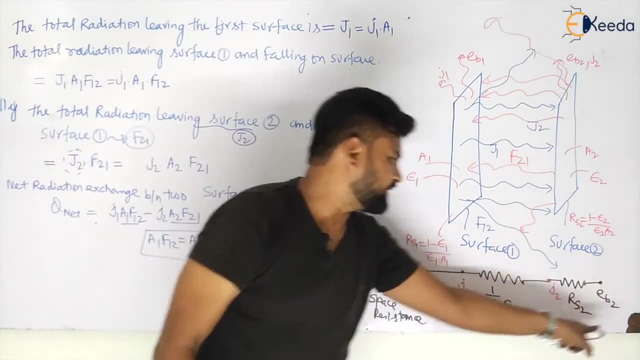 Which is nothing but this, A, B two, my dear students. and we have that is R surface too. we have that is R surface one, my dear students. So this will be the net circuit diagram for radiation heat exchange between the two surfaces. 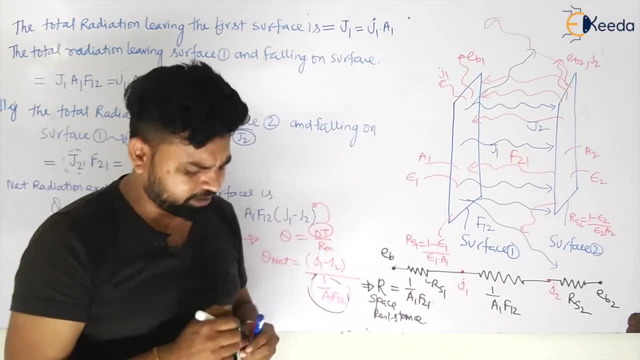 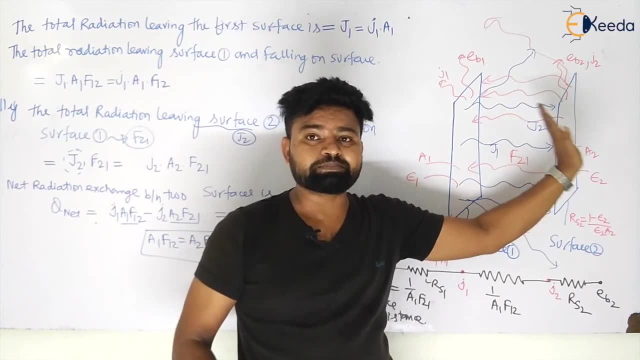 when there is a radiation heat exchange. Now let us understand the concept carefully. So if I will change the configuration, then what will happen? The space resistance will change. okay, the space resistance will change. So if I will, 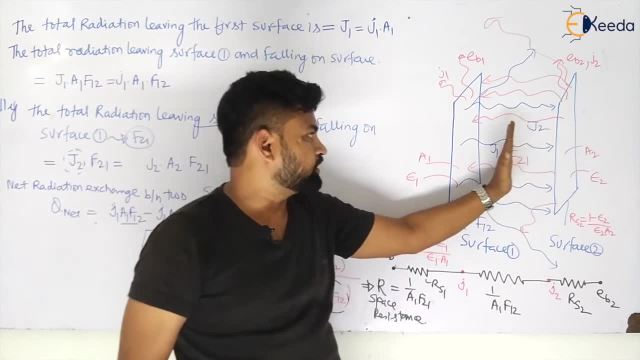 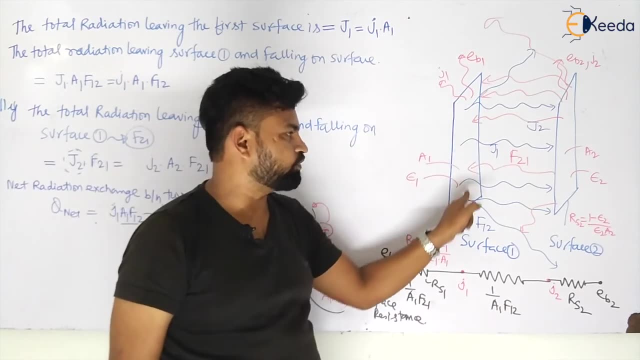 Like: bring that body closer to this body. bring that body closer to this body. what will happen? The fraction of radiation which is coming out from this or leaving this surface and falling onto will increase, will increase, and what will happen? 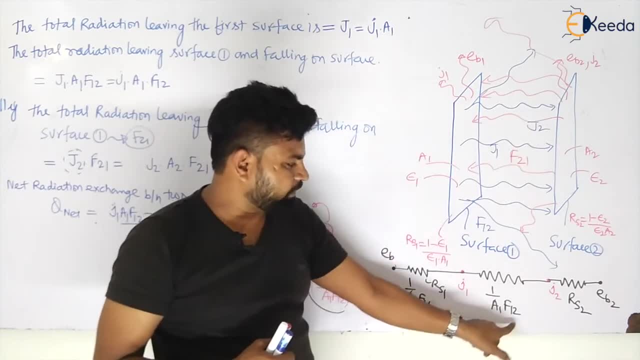 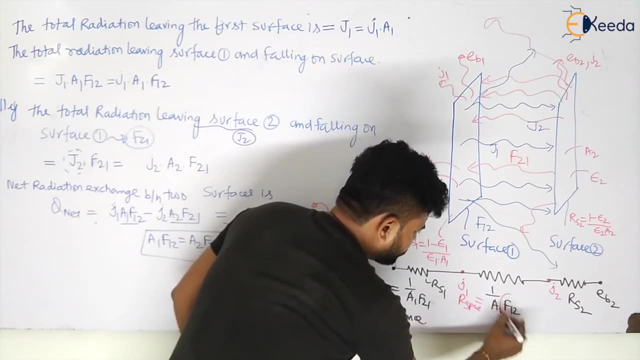 As I will bring that down. so F1: 2 will increase and due to which? due to which that space resistance, that is, R space, this will increase, my dear students, due to which R space will decrease. R space will decrease. 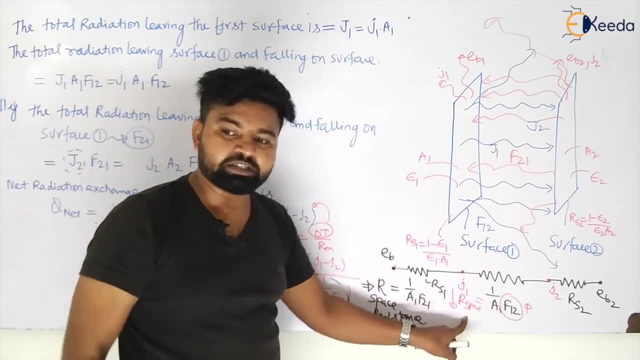 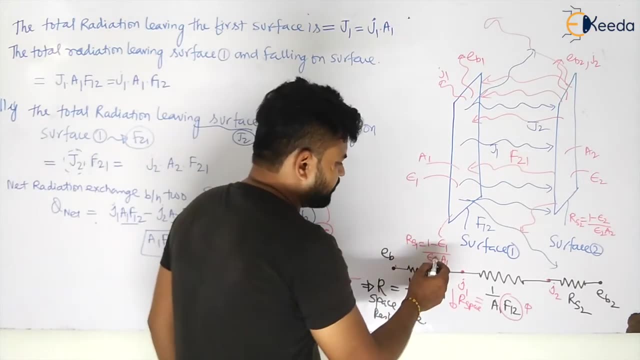 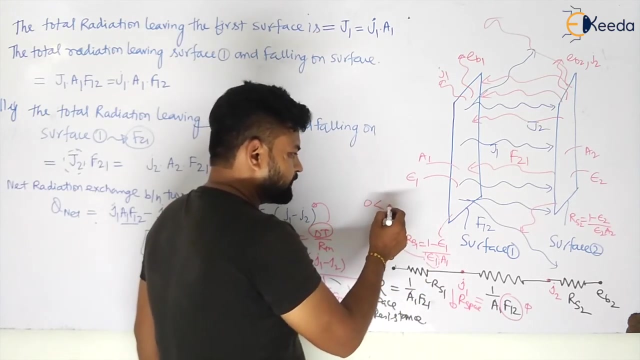 Also, if area of the body will increase, then R space will decrease, my dear students. Similarly, if, for this particular case, you will see if emissivity of the body, emissivity of the body is, is, is in the range of this, is in the range of this, that is for the 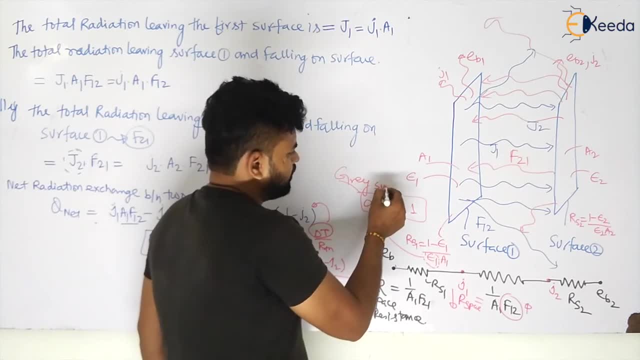 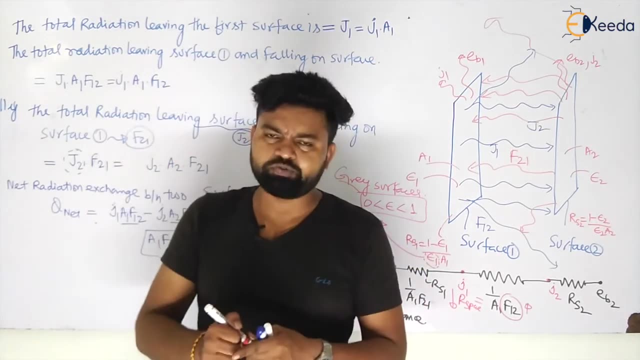 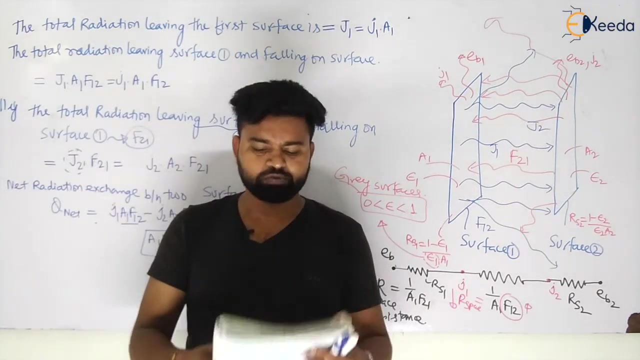 gray surfaces, that is for the gray surfaces, my dear students. So this will be the surface resistance. So now we can feel that every body, we can feel that every body, if this is your body, my dear students, so what will happen? 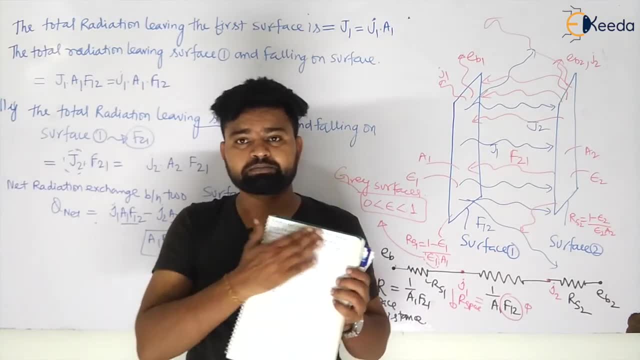 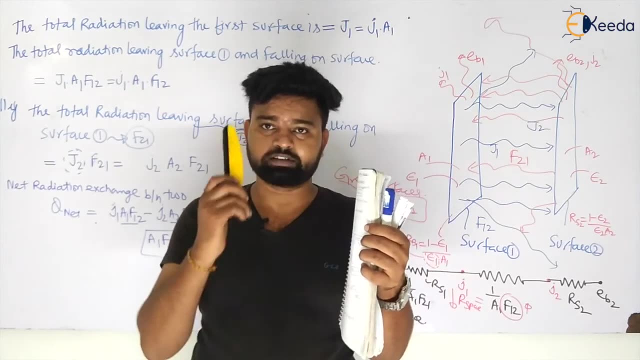 So there will be some surface resistance for this. there will be some surface resistance for this. okay Again, if this is your another body, let us say these are the another body. this is body 1,, this is body 2, and these are exchanging the radiation in between 2's. 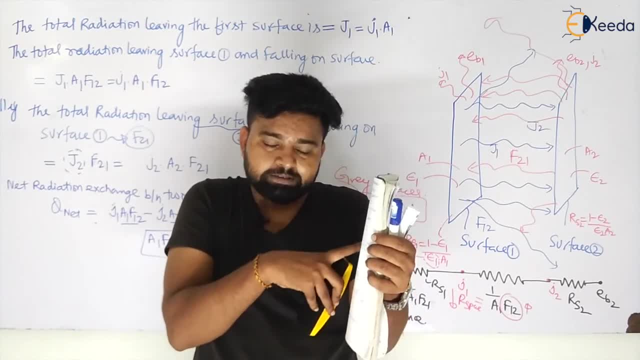 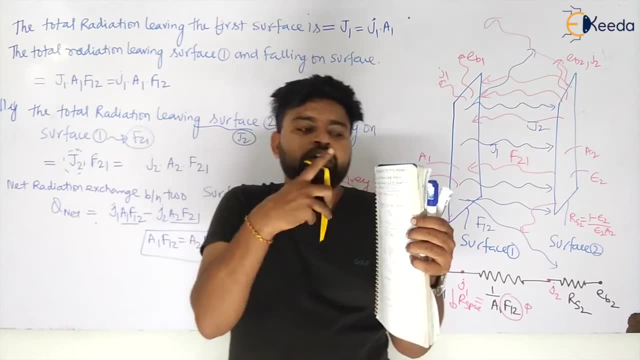 So this body- Okay, Okay, Okay, Okay- will have some surface resistance. Why? Because this surface will have some emissivity, some absorptivity, some reflectivity, some transmissivity, due to which this will have some surface resistance. Similarly, this body will also. 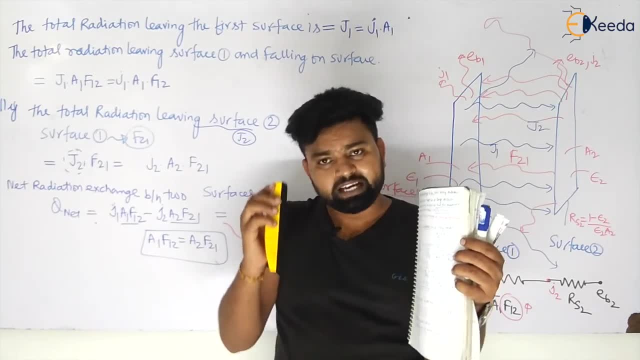 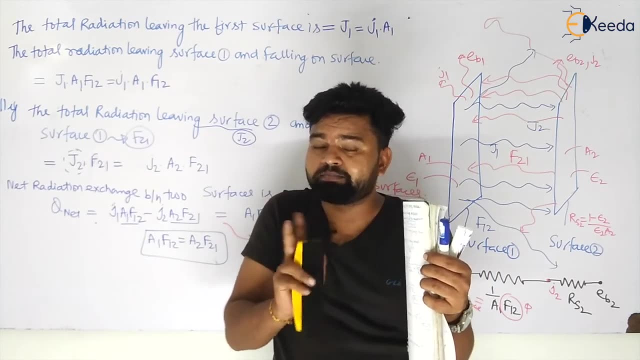 have some surface resistance, my dear students. Yes, and they will also have some resistance, which is called the space resistance. in between, the space resistance, Although the space is nothing taking nothing. but what is this? This is coming from the orientation factor or the geometry factor. So, if you will, 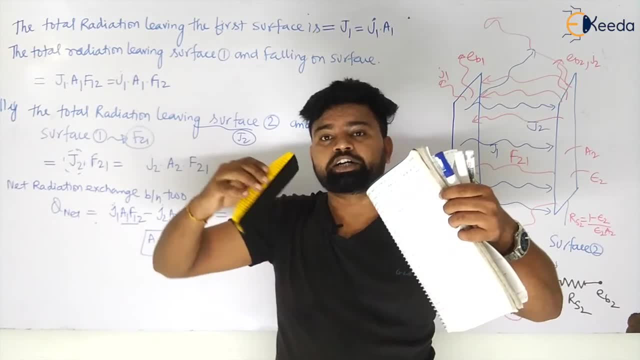 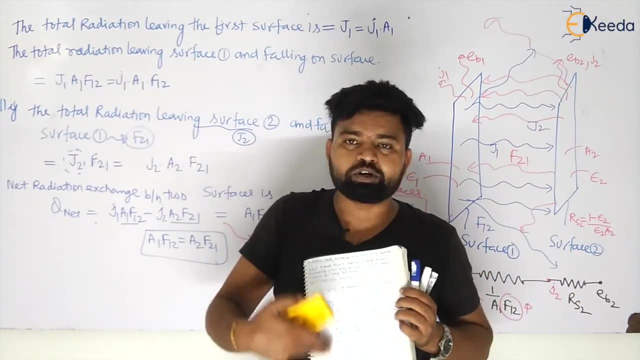 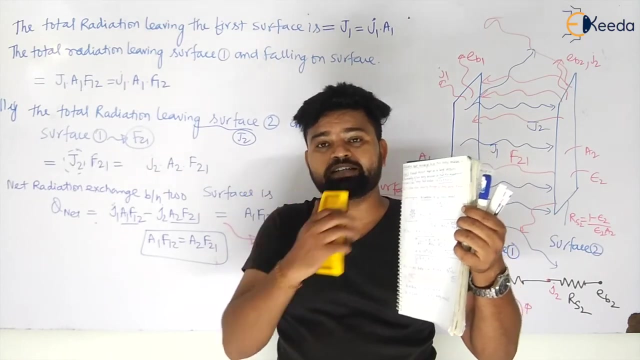 change the geometry of these surfaces, what will happen? The radiation heat exchange between them will change. Because of what? Because of the space resistance. So one radiation body will have that surface resistance and also one space resistance means two bodies. if there are two bodies, then these: 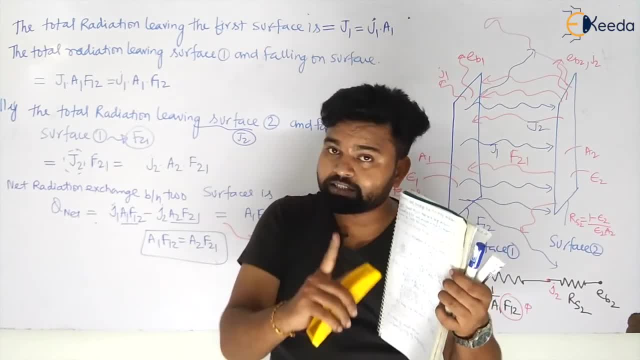 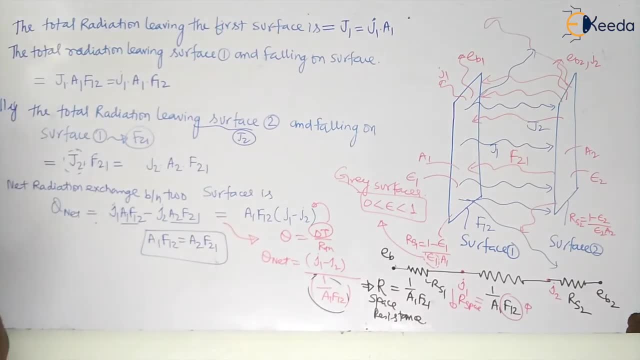 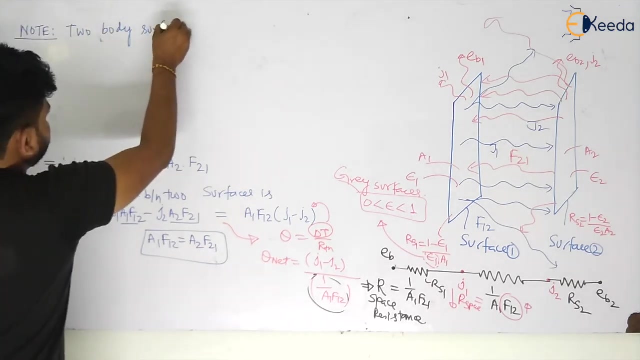 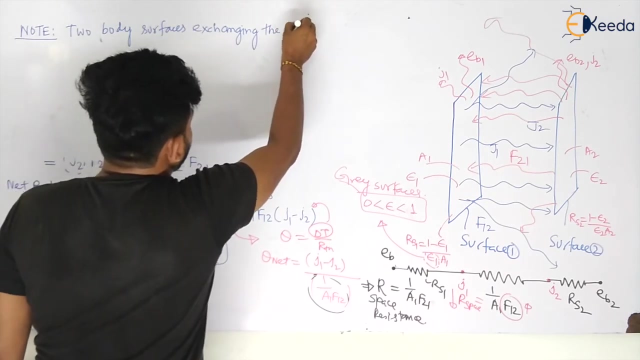 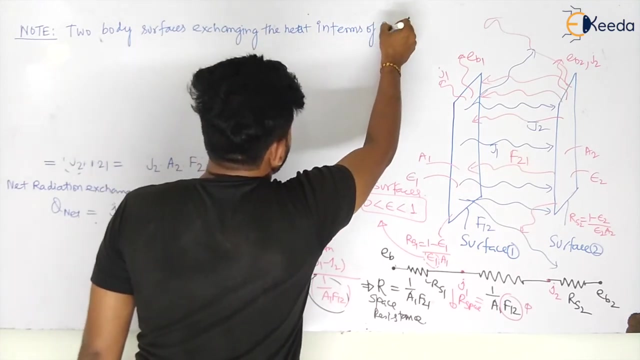 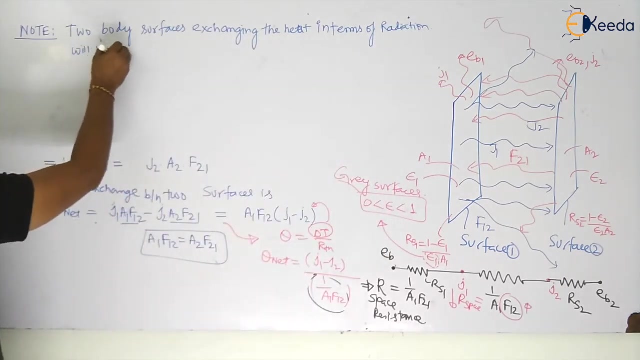 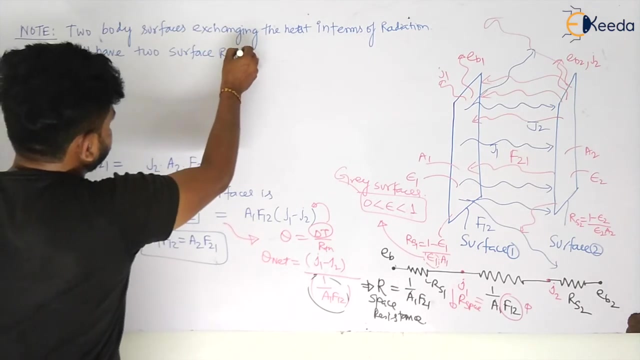 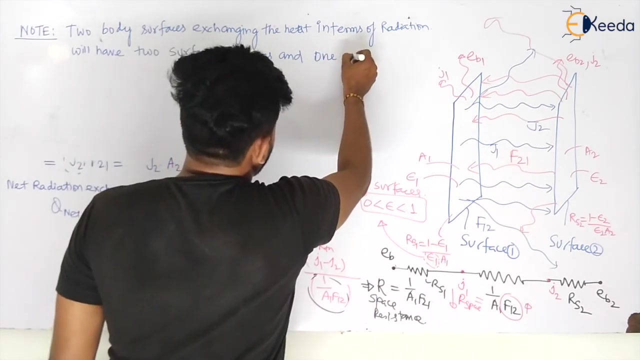 bodies will have only one space resistance, my dear students, and two surface resistances. So we can conclude now. so we can conclude now that two bodies- one body exchanging the radiation will have body surfaces exchanging the heat in terms of radiation- will have two surface resistances and one space resistance, or we also call this term as shape resistance. 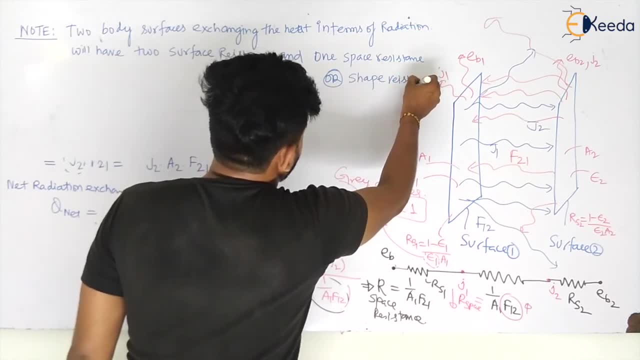 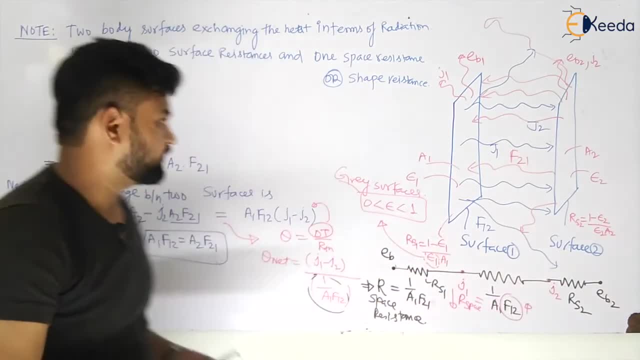 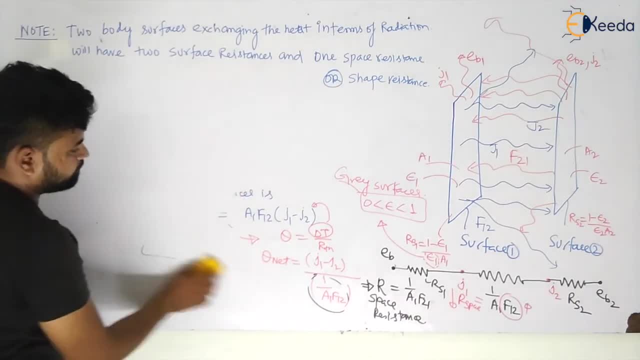 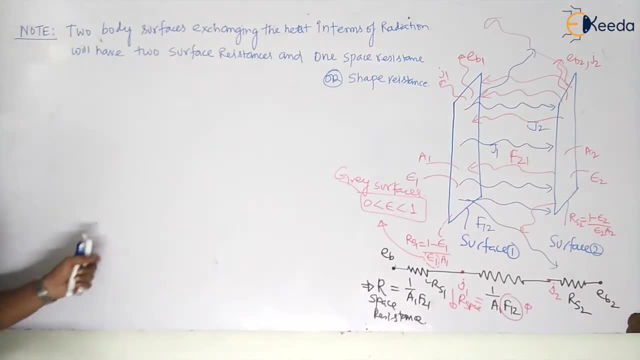 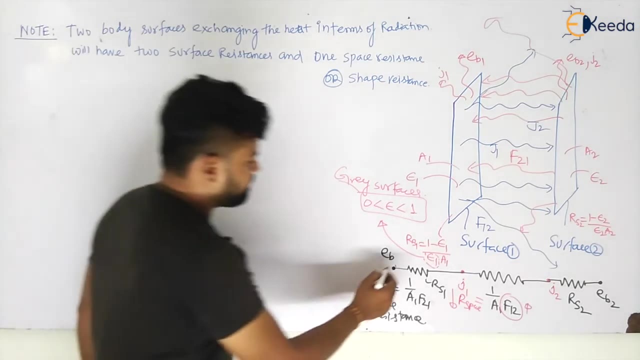 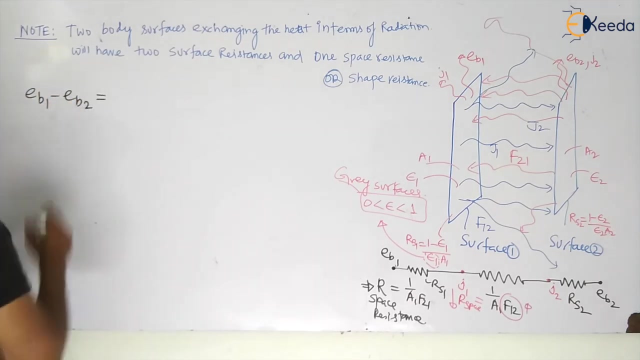 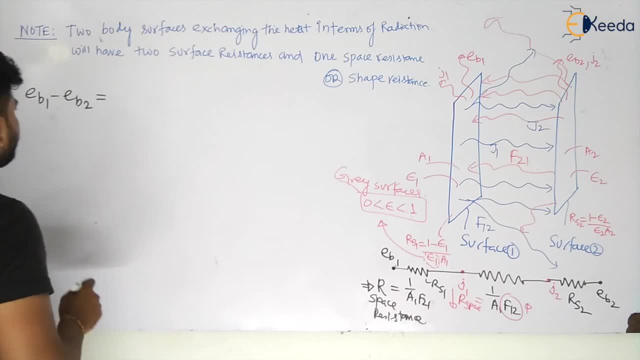 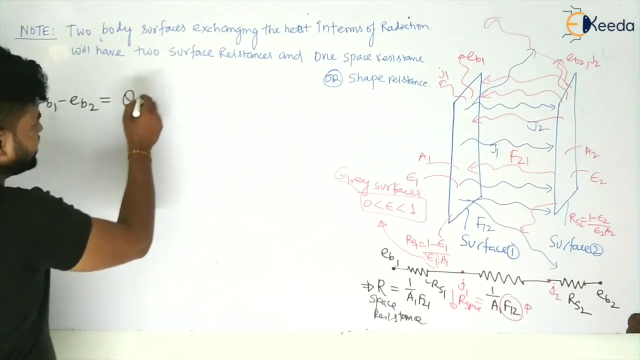 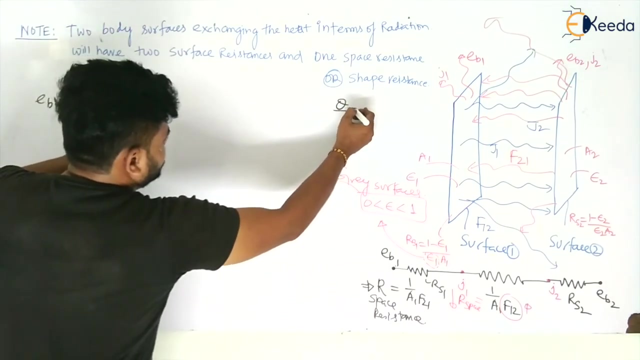 can I take directly? or yes, you can take directly. so let us write by the stage. so yes, we can take like this: AB 1 minus AB 2 is equal to Q. that is degradationaux into the effective resistance. so I have taken that Q by. so Q into R thermal is nothing but equal to delta T from this operating.